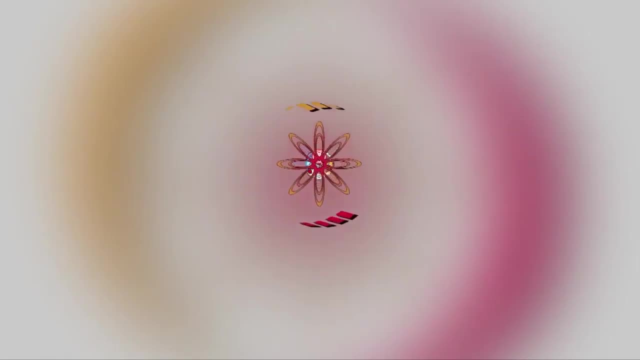 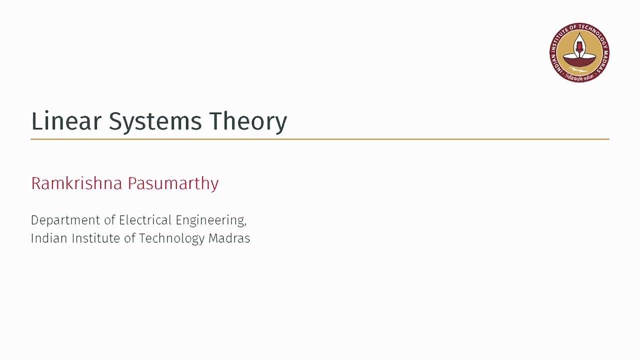 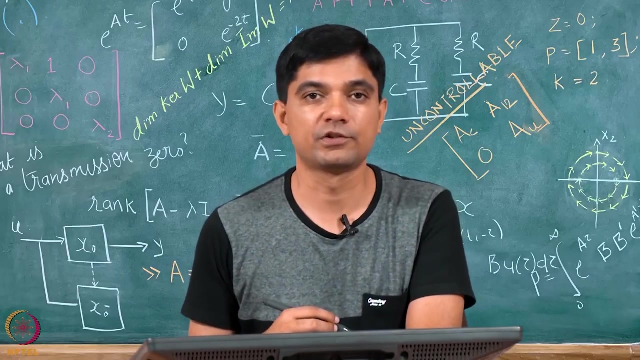 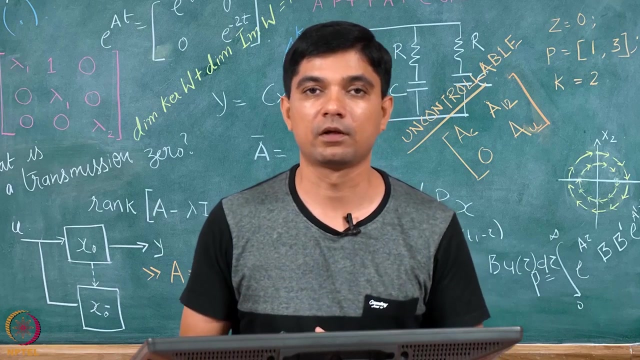 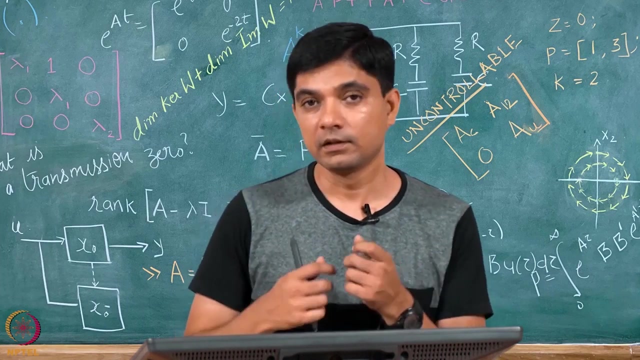 Hello, welcome to this week 6 lectures on Linear Systems Theory. So last week we had done lots of analysis about equilibrium points. We did not define properly the notion of stability, but several characteristics of those equilibrium points, via the phase space, gave us some information. 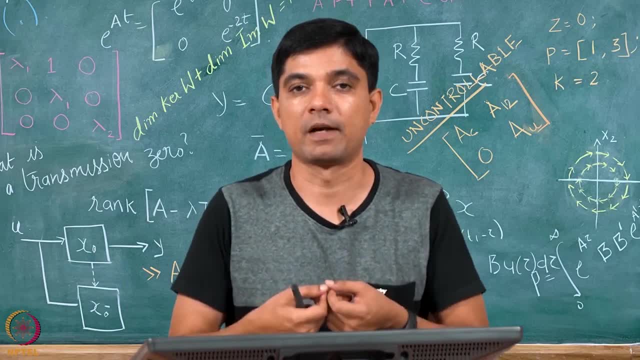 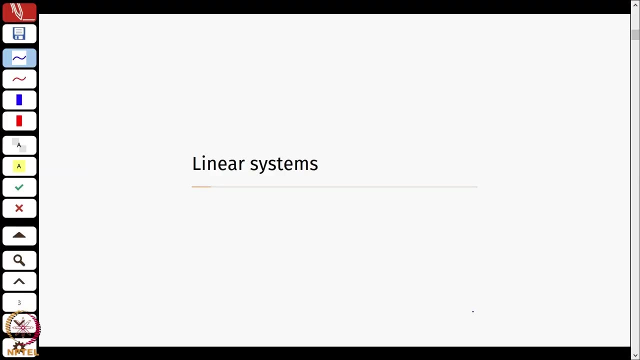 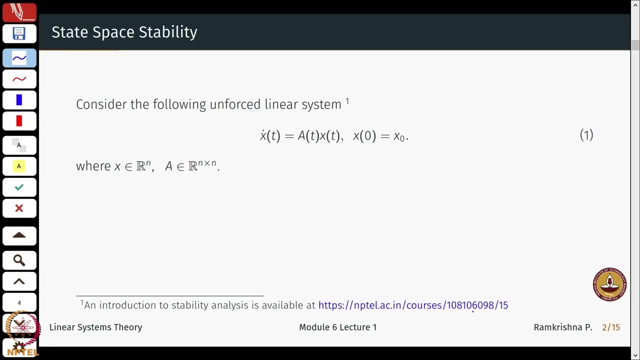 whether the trajectories around the equilibrium point were coming back to the origin or going away from the origin or the equilibrium. So today we will give a formal notion of stability. also, of course, we will do mostly in the, in the linear setting and in general in the in. 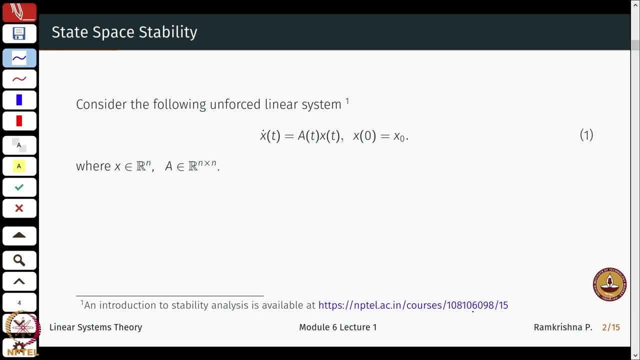 the time varying setting. ok, I will start with the, with the following unforced system and I will not talk of inputs as yet: from x dot equal to a, of t, x, t with a certain initial conditions and x is in general coming and n dimensional vector. 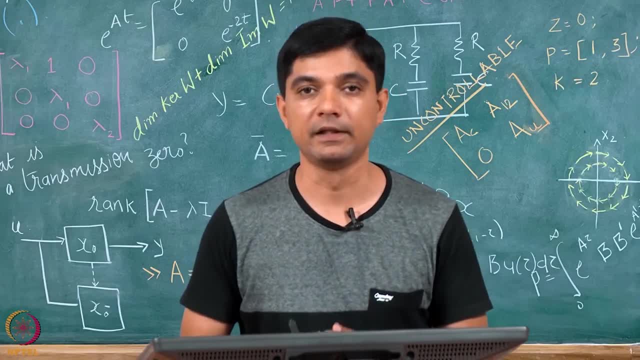 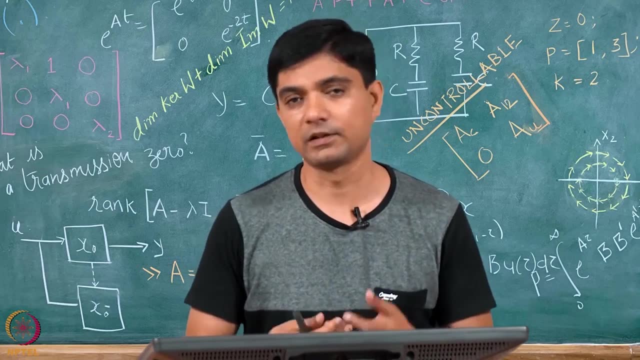 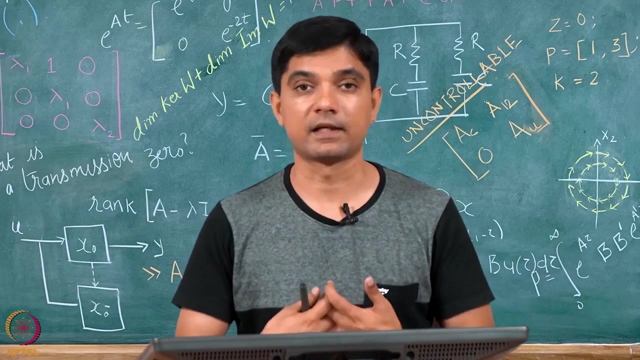 So in a control course you would remember stability, or one way of verifying stability is to look at the poles of the system. and then you had several characterizations of the poles being to the left, to the right, on the imaginary axis. repeated on the imaginary. 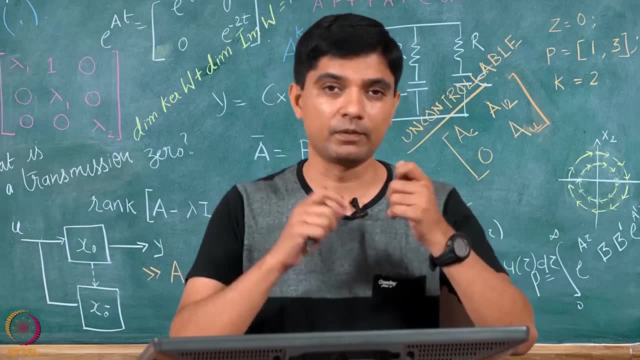 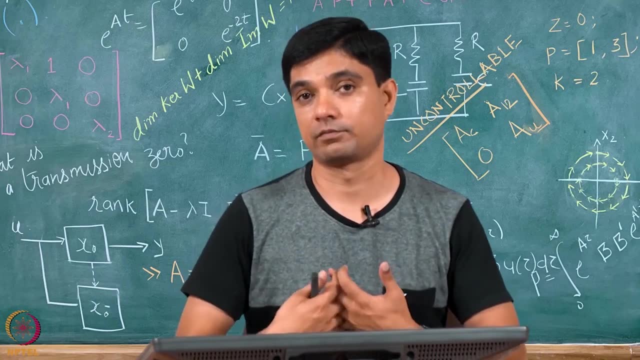 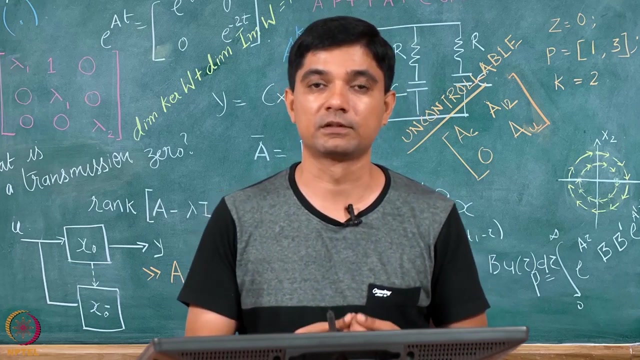 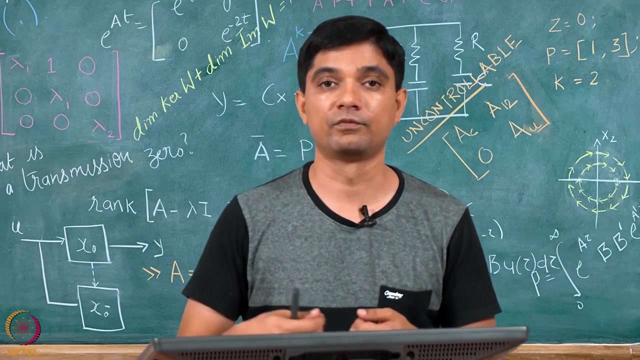 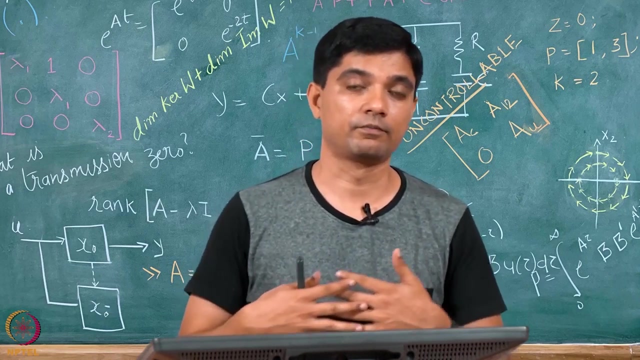 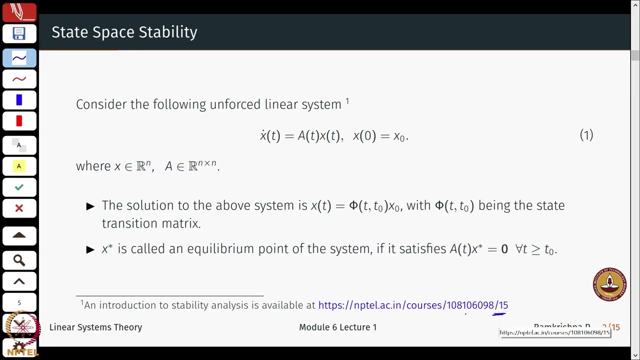 axis and so on. All this came from a bit of input, output, notion of stability right and the condition to verify or 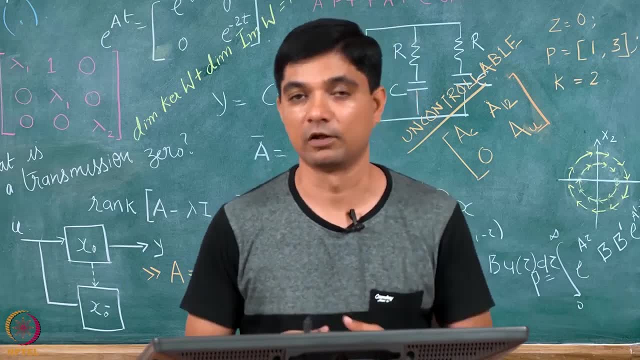 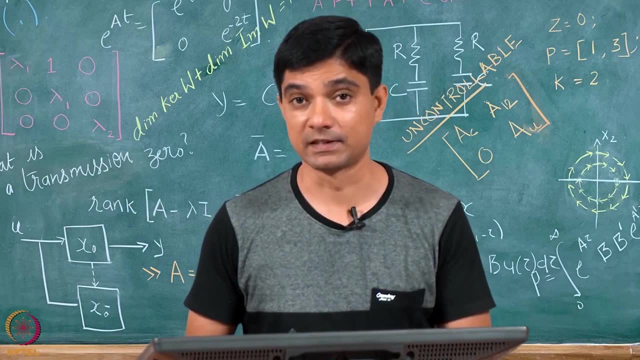 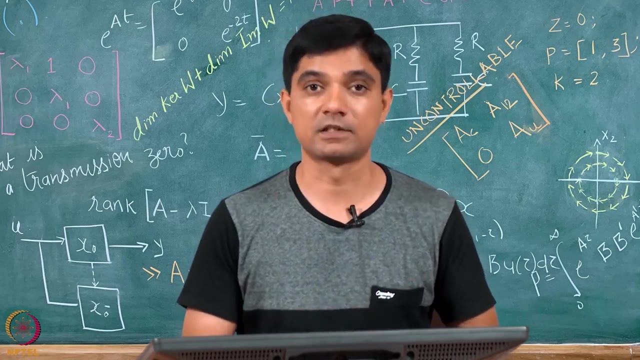 on the BIBO notion of stability, of what was the bounded input, bounded output notions of stability. I will not elaborate that. but here what we will essentially focus is on the state space stability, more related to the kind of solutions we computed for the 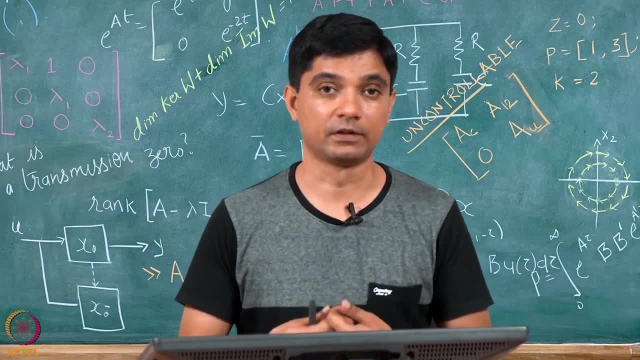 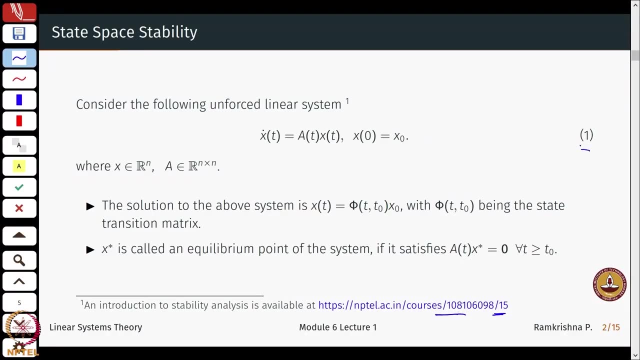 system of linear equations, starting from the concept of a state transition matrix. ok, So for this class of systems, what we know is that the solution is well given by x, of t is phi, which is the state transition matrix and an initial condition. What we also know, 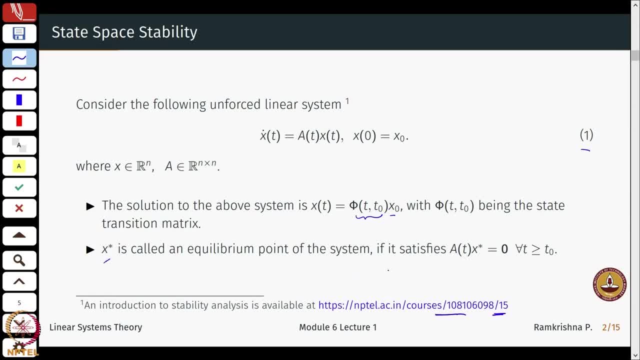 is that x star is an equilibrium point of the system if it satisfies A x star equal to 0 and in most linear cases the- you know the origin x star, The 0 vector, is an equilibrium. it is always, even if the A matrix is not invertible, say: 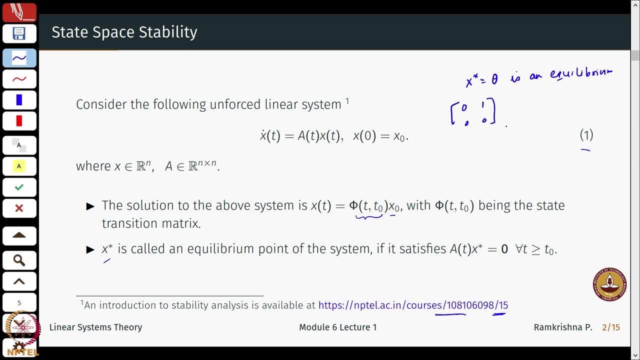 if it is of this form, still, 0 is an equilibrium. There could at some point of time be well multiple equilibrium. say, this is an equilibrium point. the origin may be somewhere. this is also equilibrium point. I think these two points is also will any point between these two points or the straight. 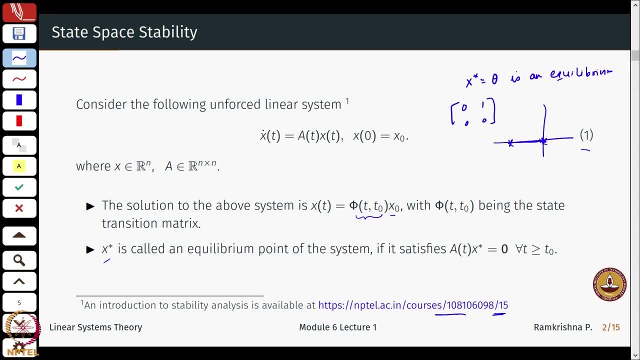 line joining these two points will also be in the equilibrium. ok, So you will have essentially an equilibrium subspace. that is what we talked about in one of those conditions in equilibrium in previous weeks lectures. ok, So fairly we will just generally denote the notion of equilibrium as x star and mostly. 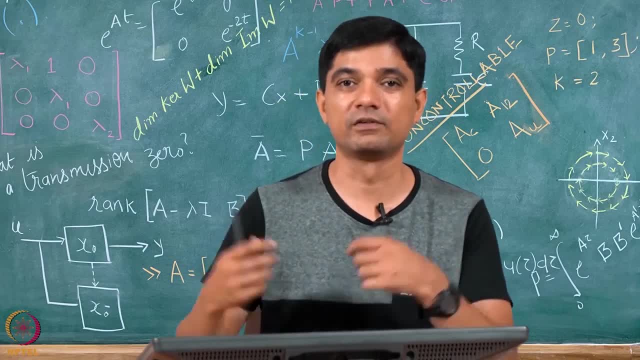 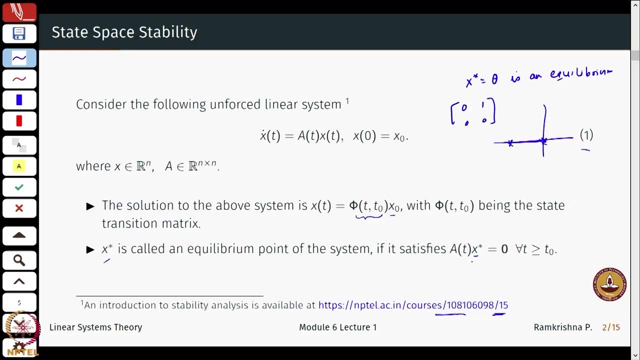 we will deal with the origin. Even if the origin is not the equilibrium, you can shift, change the coordinates or shift the origin Slightly different than the non-linear case, because there we possibly will not have an equilibrium subspace but we will have, say, isolated equilibrium, point, say equilibrium. 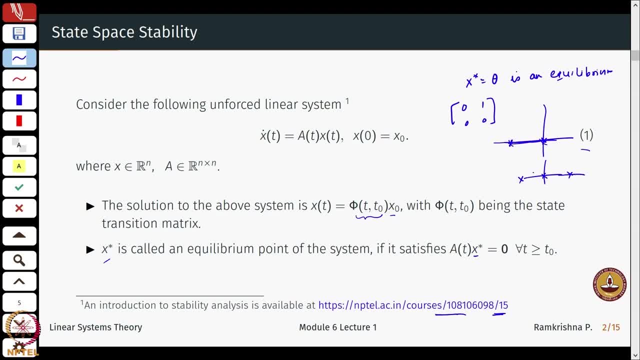 point here, equilibrium, point here, here, and so on, And each say: if maybe the phase space goes something like this, sorry it could go this way, right this and this. So this is a stable equilibrium. these two equilibriums could. 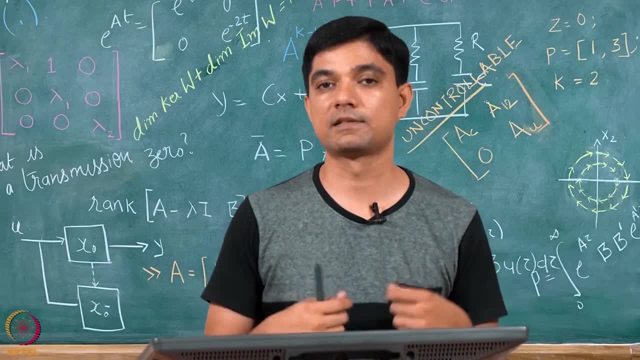 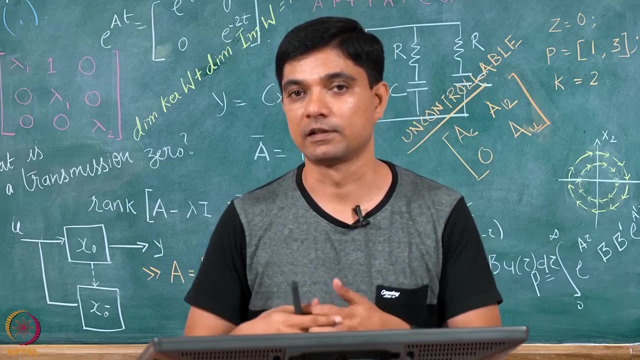 be unstable, and so on. So we have what they also called as isolated equilibrium points. but for us we will just assume that, or we know that origin is the equilibrium and that will be the equilibrium of interest. but just to, for notational purposes, we will just call: 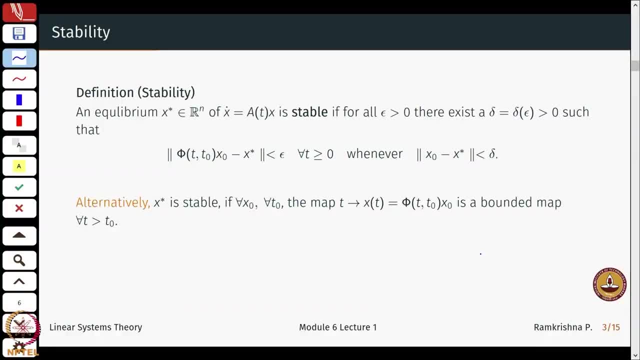 it generally as x star. ok, So the first definition of stability. what does it mean? Again, I am looking at, stability is always defined with respect to an equilibrium x star. So an equilibrium x star of the system x dot is A, t, x and I. just for ease of notation, 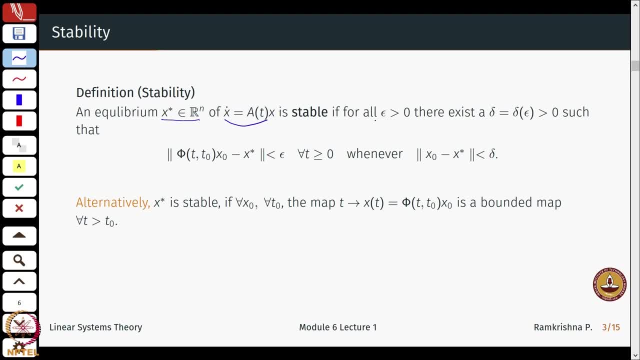 I just drop the time argument, for x is stable if for all epsilon greater than 0. There x is a delta which is a function of this epsilon, such that, if I take the norm, So this is a solution right, how the solution trajectory moves, phi, t, t, 0, x, 0 will give me: 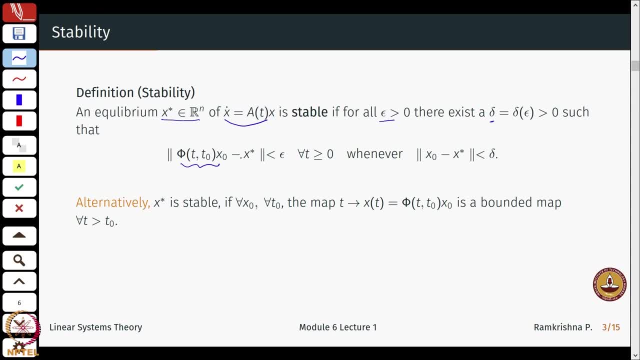 the solution. The norm of this solution minus x star is less than 0, whenever x 0 minus x star is less than delta. ok, We will come to this right. where does the epsilon come from? where does the delta come from? In some cases, you also have the. 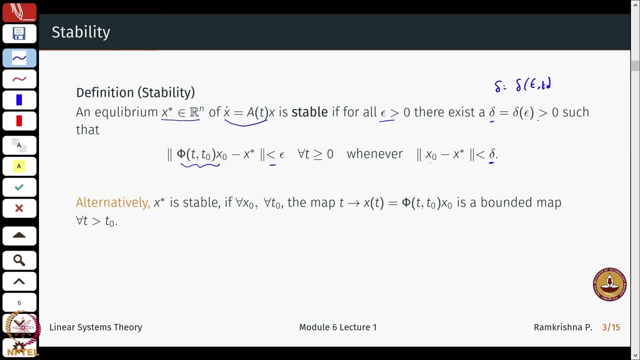 Where the delta is depending on the initial condition, and in this case it is not depending on the initial condition, So it is usually called as the, also referred to as the concept of uniform stability. ok, So we will drop this, t naught for the moment and we will say: 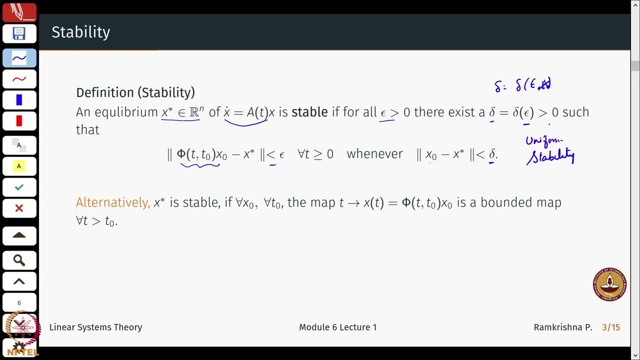 well, this, we are just dealing with: uniform stability. ok, A slightly milder version of this to give an intuition of what this statement means, or a little understanding of this. So we will come to this right. where does the epsilon come from? So we will come to this right where this definition means, or a little understanding. 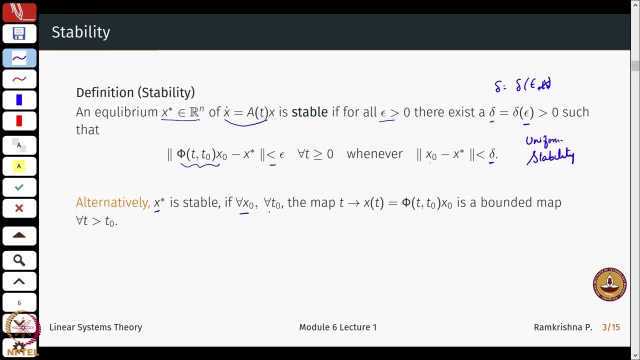 x star is stable if, for all initial conditions, for all initial times, the map t from x, t right, which is given by the solution- This is my solution- is a bounded map for all times t greater than or maybe even equal to t 0. Essentially it means that phi or this solution, x of t. ok, So it is a bounded map. so means: 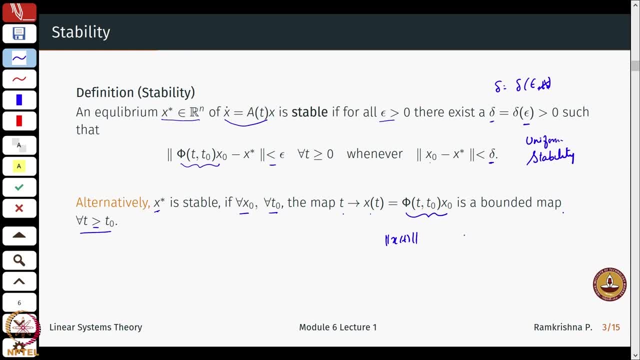 the values of x never go unbounded. So if I were to just draw a little picture, this could be solutions, whatever, and so on. right, So these are all bounded. ok, Now, what does what does this actually mean? ok, So let us see a pictorial version of it. So I start with x star, as 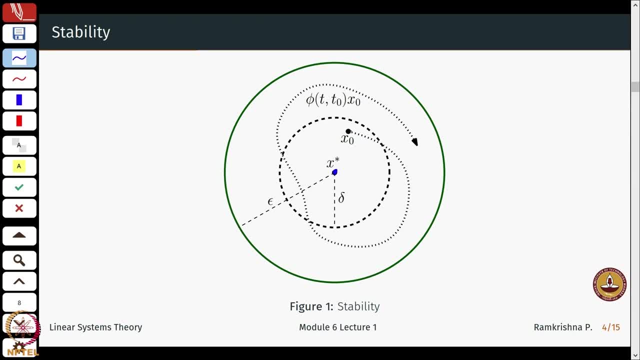 my equilibrium point here. Let this x naught come from a delta ball. essentially, delta ball would be a ball centered at the equilibrium and of radius delta and take any initial condition. So I have this delta ball and take any initial condition within this delta ball. this x naught. 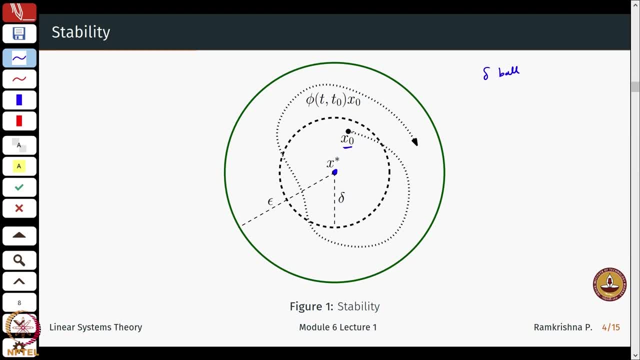 So the solution will. so if I just see this dotted line, the way it goes, it is always conformed fine to this epsilon ball of radius. you know this is epsilon ball is again the ball centered at x star and of radius epsilon. ok, So if I just move this picture 90 degrees, it will. 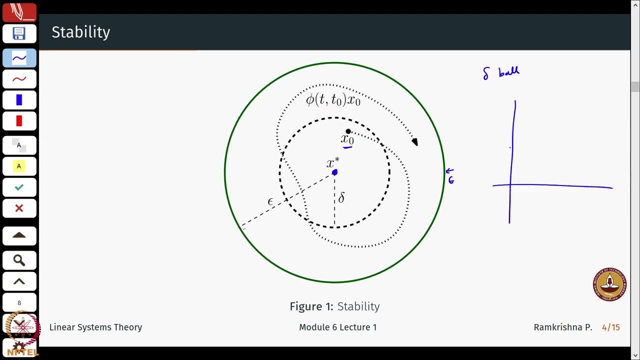 look something like this: ok, I will try to draw it as neatly as possible. say somewhere: I will just use this red color for the delta ball. So this is my delta ball. Ok, And I will come back to blue. So what does this mean of I start at some initial condition? 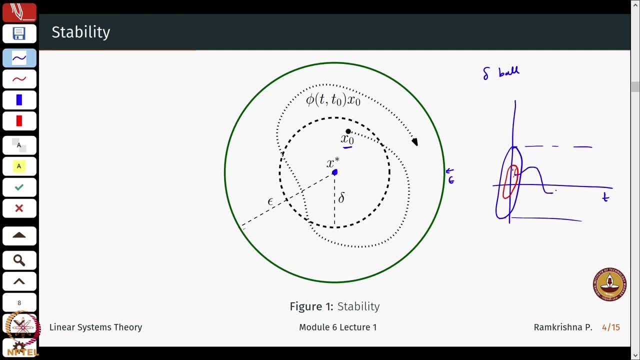 here and as time goes by, I am just within. the solution is just within this cylinder. it could be: go here, go here and so on, but it will never bridge this cylinder right, So it will just move along the cylinder. So here I am, actually even adding the time. 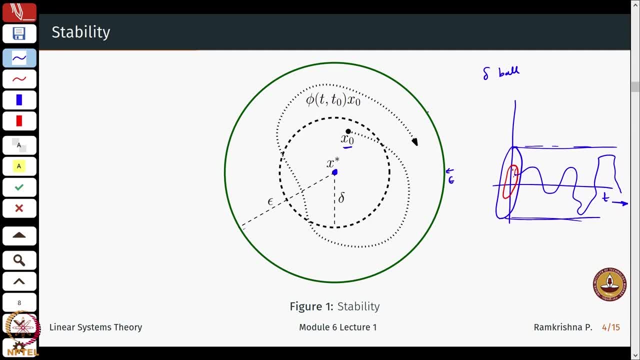 axis if I tilt it. So these solutions will just move along this cylinder which is in this, in this represented in green. So essentially it means that the solutions do not go like unbounded. So for example, if just say I started initial condition here, 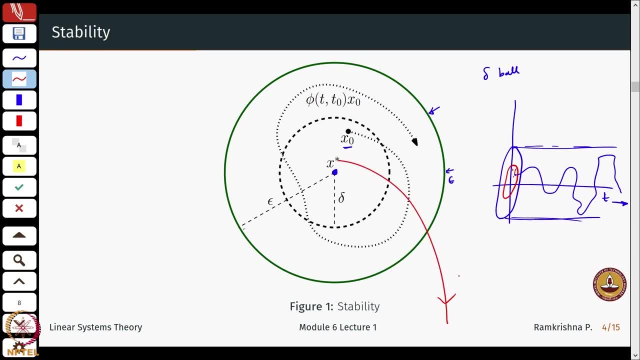 and just keeps going this way. this is an unbounded solution and this is an unstable behavior, right? So this is a very basic, very weak notion of stability that this could just be whatever. the solution could just be doing whatever they want. One simple example is: 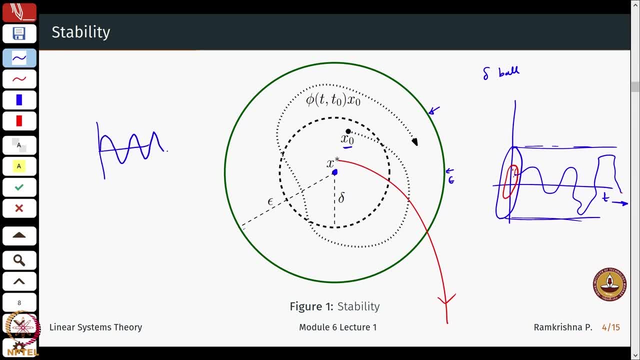 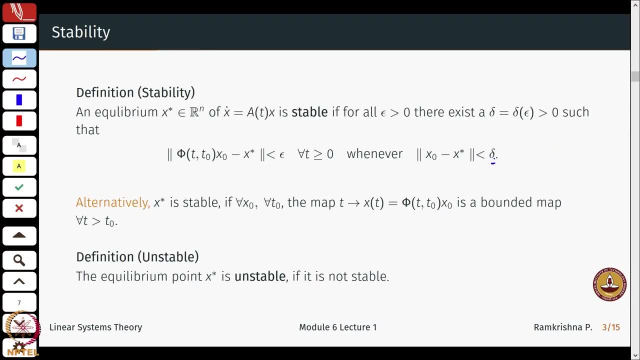 the linear oscillator that we did right. So it just keeps on oscillating this always stable, right? ok, So that is what this says, right? So whenever the initial conditions are in a delta ball, the solutions will be confined to an epsilon ball, or that the solution, or 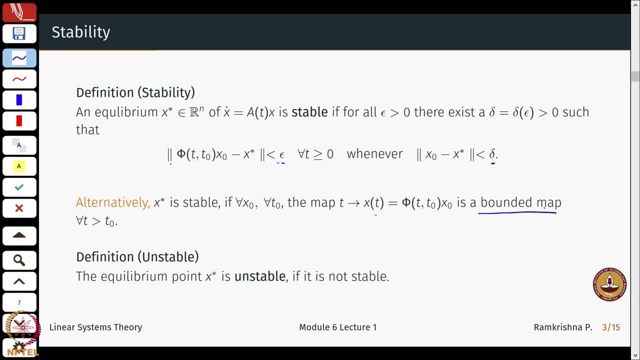 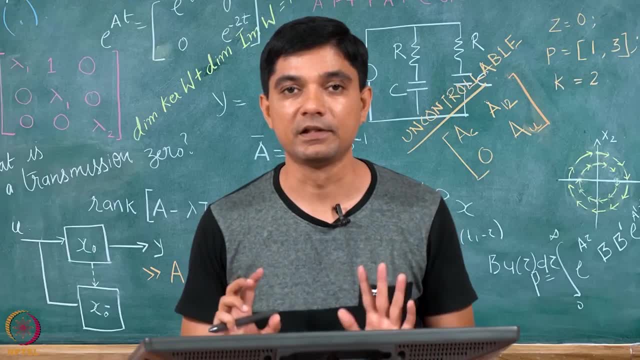 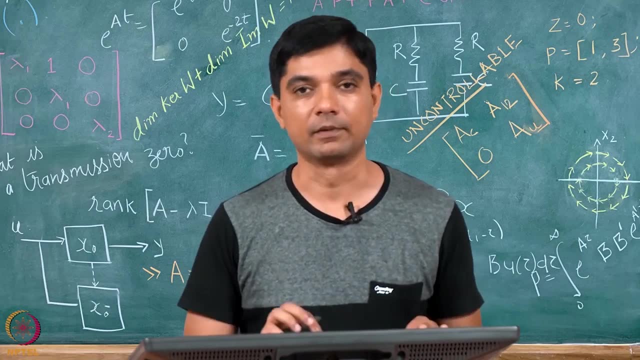 this map t to the solution. space is always a bounded map right. That is what is a very loose, or the basic definition of stability. what is unstable? there is only one definition: whatever is not stable is unstable. So that is the only definition of instability. You 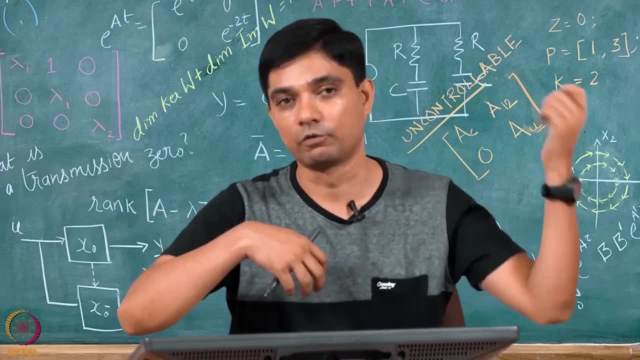 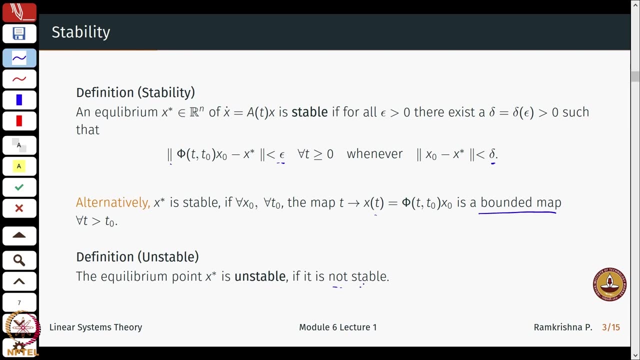 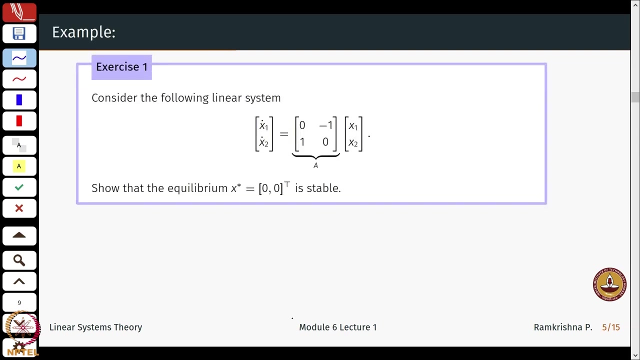 do not really check out the solution going to infinity, or the doing whatever and so on. So whatever is not stable is unstable. ok, So that is the only definition of a system being unstable, ok, So just to give you a little, very basic. 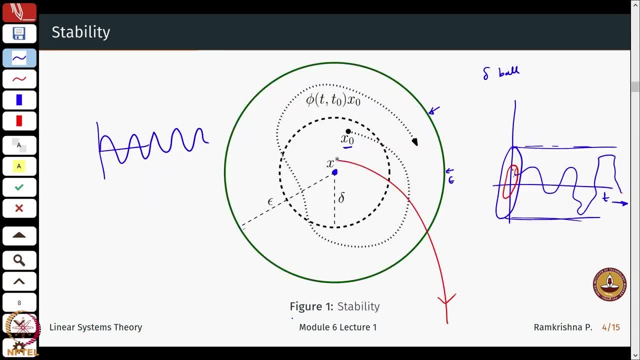 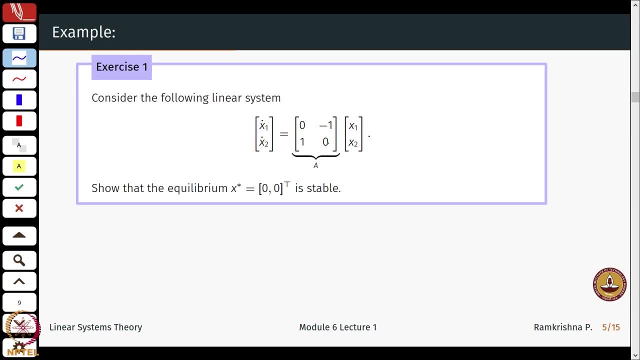 basic, seemingly trivial illustration of what is happening in this picture. So let us start with this second order system: x 1 dot is minus x 2, x 2 dot is x 1, and so on. Show that the equilibrium is stable, right. So easy to verify that 0 comma 0 is an equilibrium, ok. 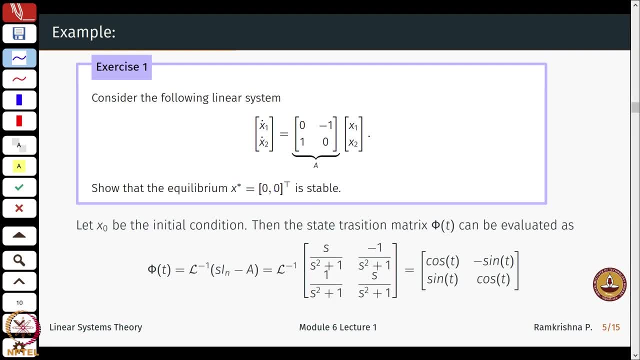 Let us first compute the solution right and just let us, for simplicity, assume that the initial time is 0. So let x naught be the initial condition. there is a state transition matrix. well, we know how it is computed this way. I do not. I will not go into the steps. 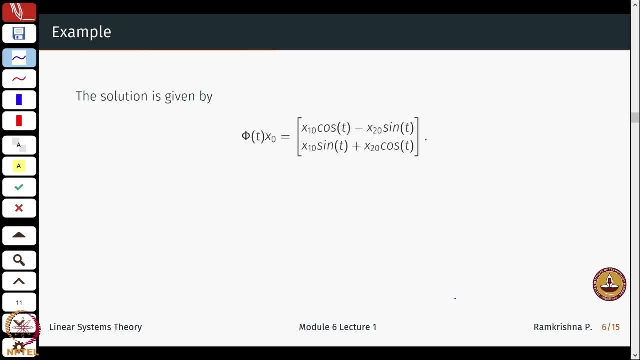 of this, but by now we know how to compute the state transition matrix. So, given any initial condition- x naught, which is a two dimensional vector- x 1 naught or x 2 naught- the solution will look something like this: ok, Now, given x star, which is just the origin, 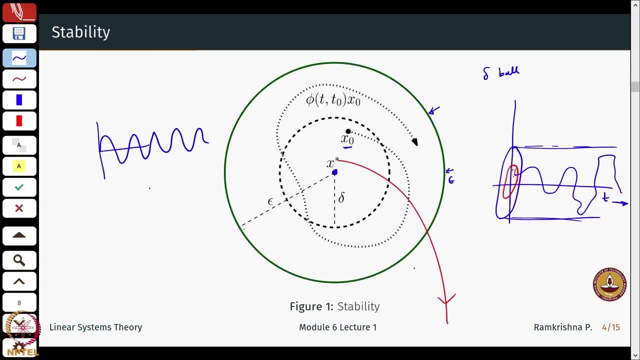 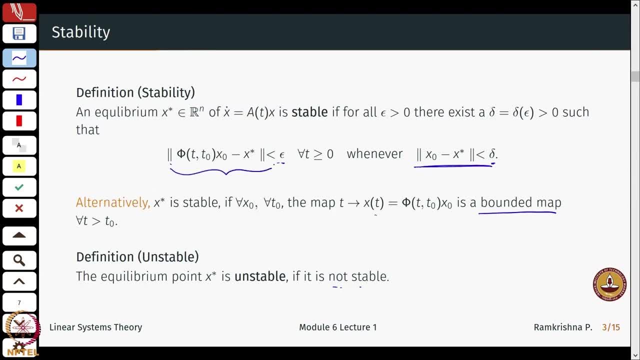 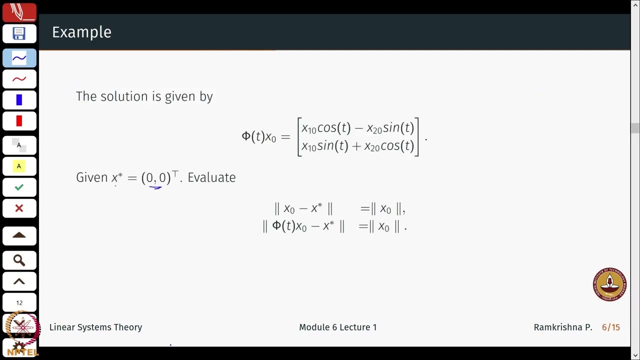 matrix. what I would want to evaluate is: checked for these two inequalities right, If the initial condition is within a delta ball, or the solutions within an epsilon ball, or all the solutions always bounded. ok, So let me compute this norm right? So this: 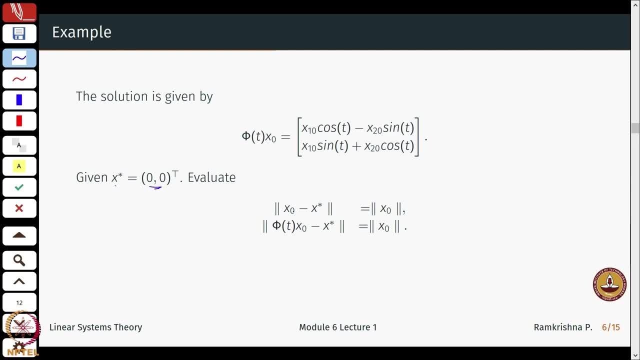 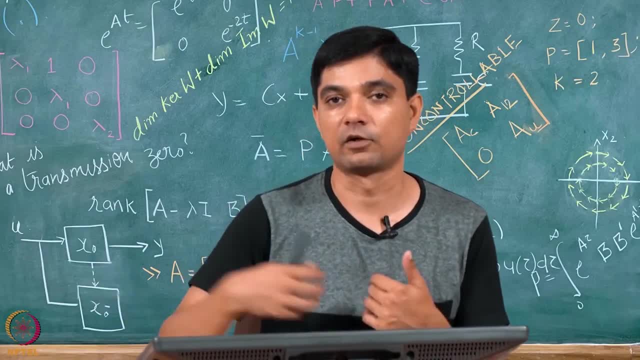 could be two norm or infinity norm or whatever, because we know that all norms, infinite dimensionals, are equivalent. So give me one norm, I can always find a nice relation with the other. I can always bound it with the other norm. So it does not really matter which norm you 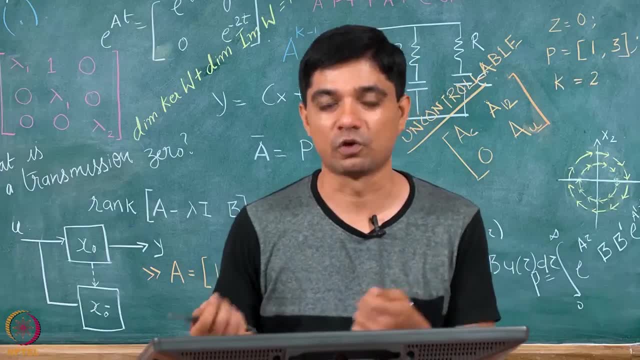 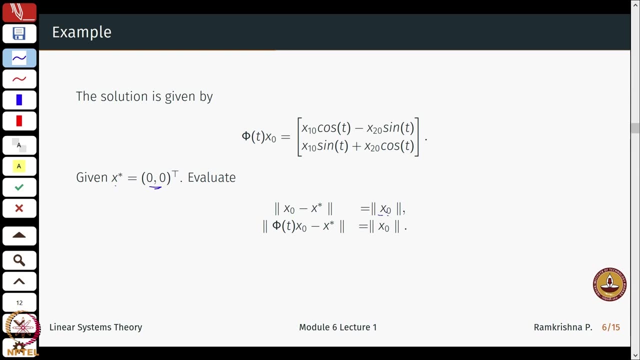 choose, but for our purposes we will usually look at the two norm. ok, So this. well, x star is 0.. So this turns out to be just x naught. ok, Now the solution: phi, t, x naught minus x star. So this is. computations become easy, right. So if I evaluate the two norm of this, 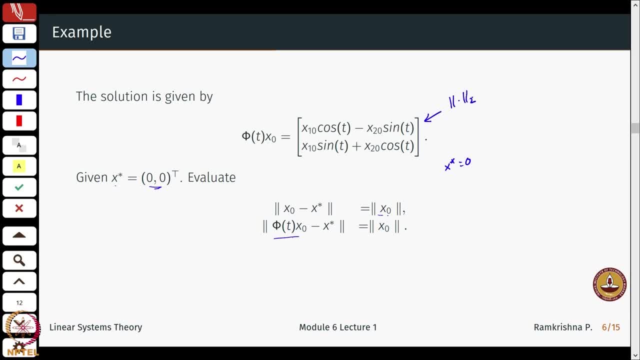 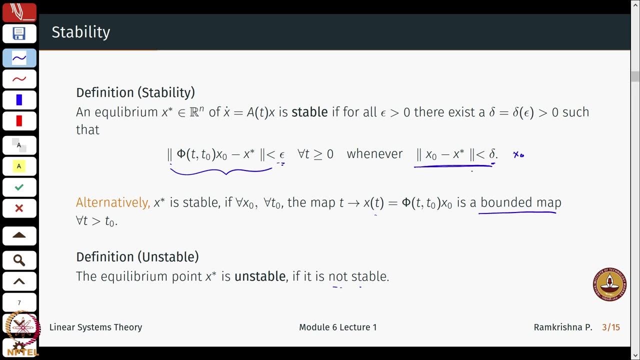 solution: ok, It again turns out to be x naught. ok, So what does it mean? is that? well, the initial conditions, So the delta, So this: I found a bound to be x naught, or actually I found it actually to be equal to x naught. this is: 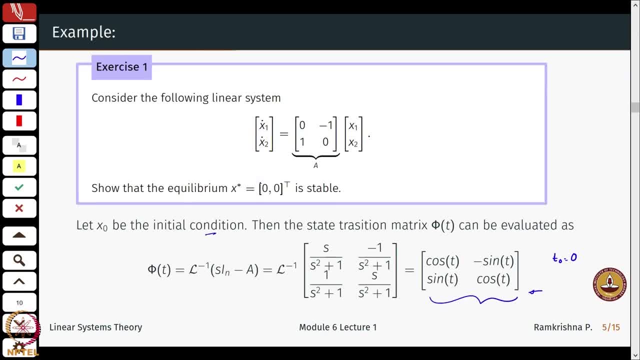 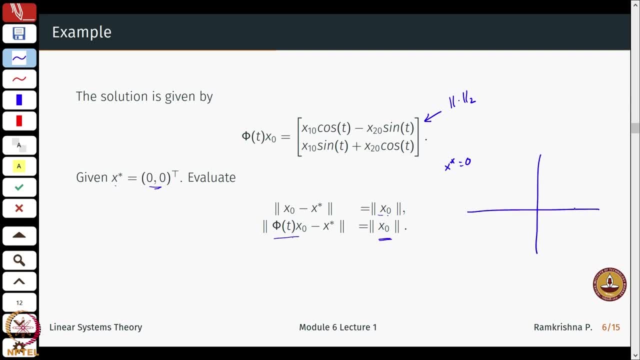 also x naught, ok. So let us take a trick to verify or to understand what this means. What we know is the phase space. the phase space of this systems are concentric circles. So let me say I take this initial condition: x naught So. so this will be my delta ball. 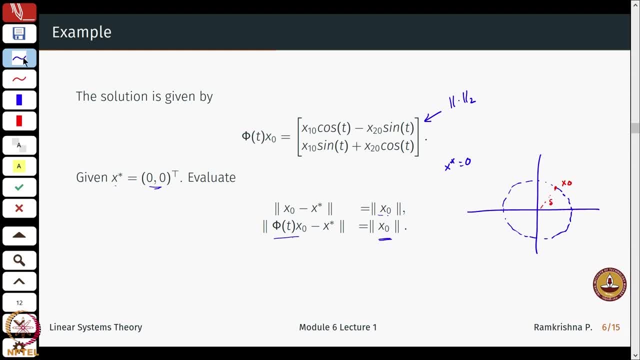 ok, Now where will the solutions move? Well, the solutions will move along this circle of radius, delta, right along all this. Now, this is also equal to epsilon. that is what. that is what I mean when I draw these two pictures. right, I start with the initial condition. 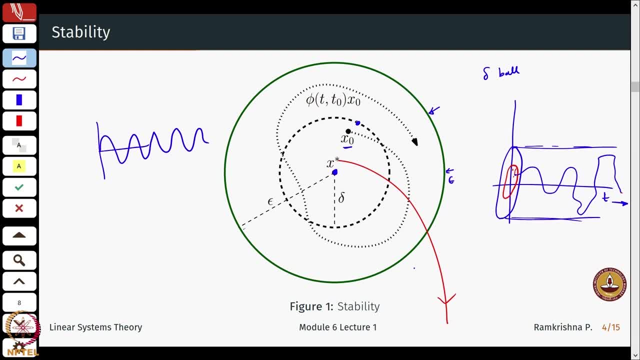 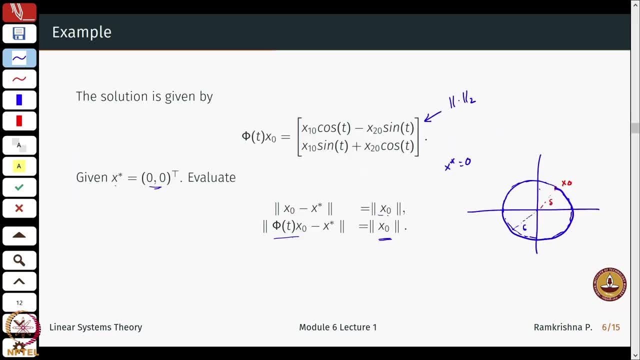 So we will give x naught 0, this will be y naught, okay, So this is what we will be putting at this point. So this is, whatever is my initial condition. then the final conditions will also be- or the solutions will just be circling around this again of the same radius. 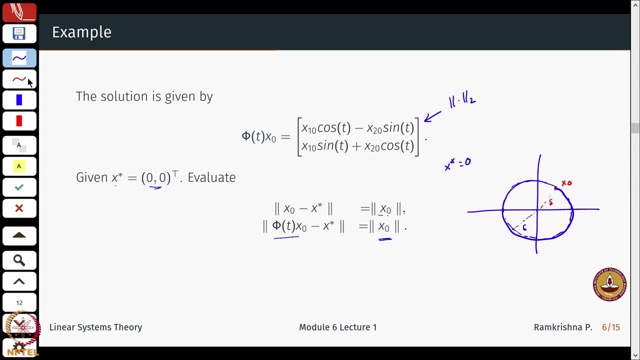 Further if I say, what if my initial condition is here? So I will have a new delta, let me call this delta prime, and my solutions, starting from here with some initial condition, will just be circling around here. ok, So they will never go unbounded, right? So that is. 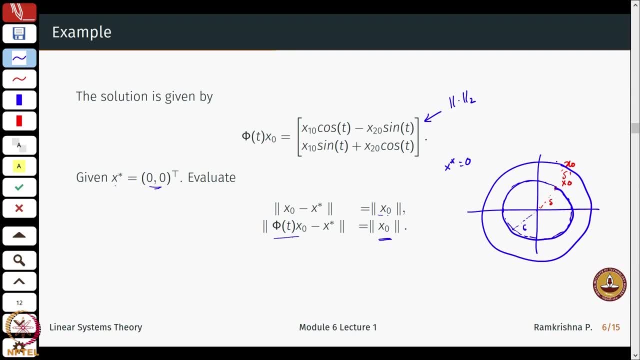 the. that is the. that is the idea here. So I can just say: take a larger ball like this, start from my initial condition here, and they will actually. the solutions will just be inside this. ok, So very, very nice and a trivial example, but it gives us a nice understanding. 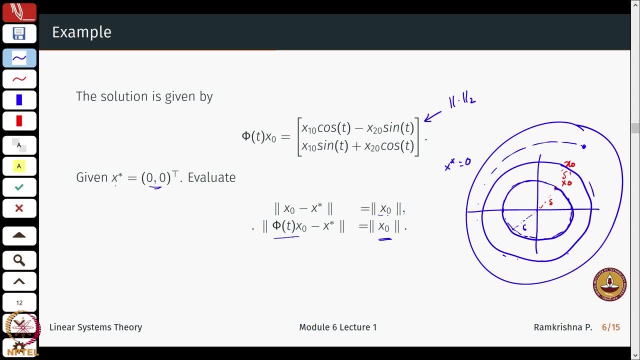 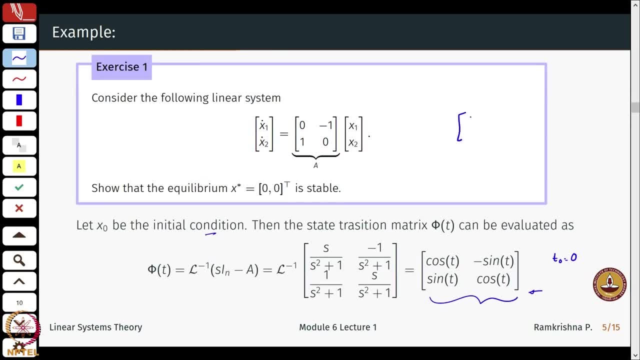 of stability. It is easy to check that this system will have complex eigenvalues and so on. As a exercise to check if the system is or or an example for instability, just check for this matrix and then try to compute the epsilon and delta values and you will find that this will not actually not exist. So you will. 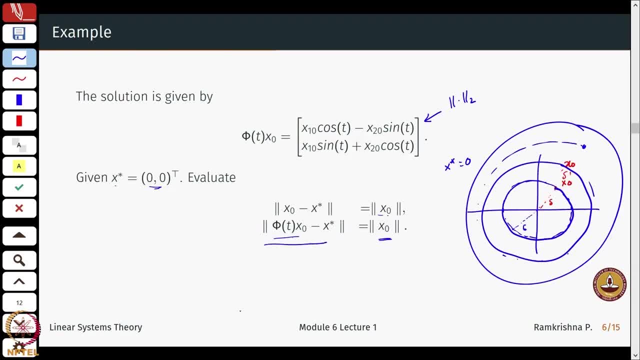 not be able to bound this by some number from the above. ok, So I will not not really do that example of instability, because that it should be easy to check and this is like what I proved here is: I can just check that for every delta greater. 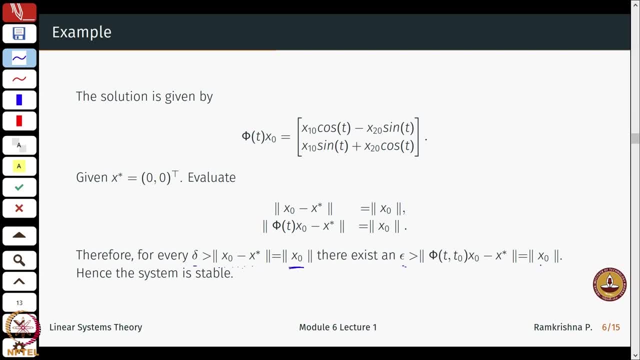 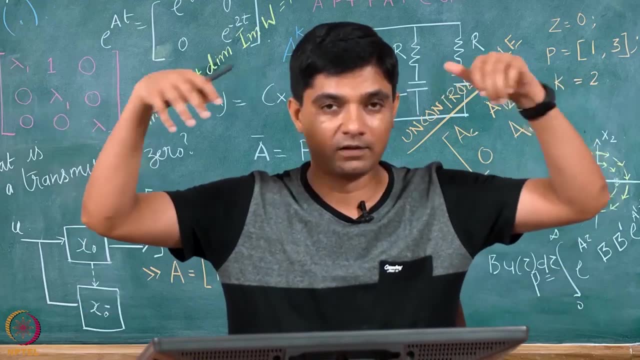 which is x naught. there exists an epsilon which is x naught, and hence the system satisfies the definition of stability right Now. what next? I really do not want systems which are- I really do not know where they are going, but they are just bounded. I want. 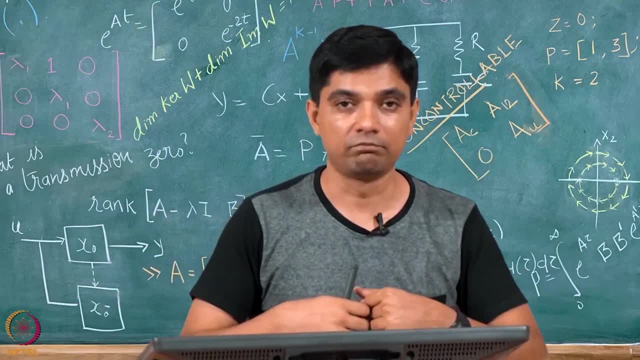 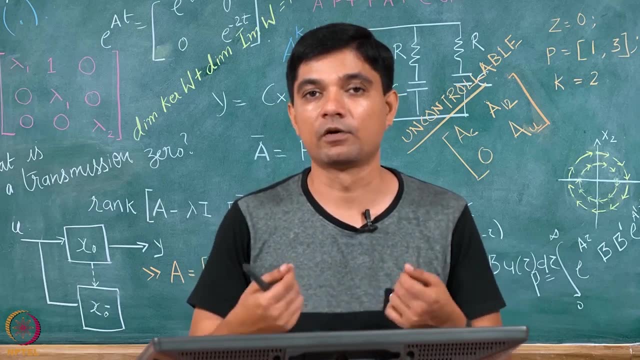 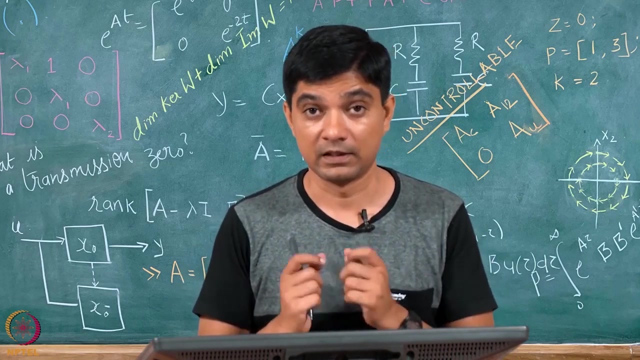 something stronger, right? So stability. I would rather want my system to come back to its equilibrium or its steady state position when it is subject to an initial condition or there is a slight perturbation in the system. Now, how do we mathematically define that? 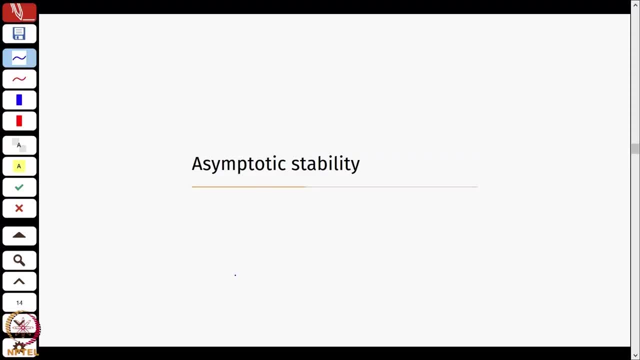 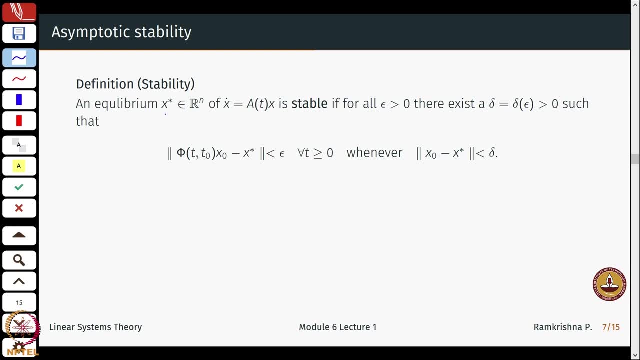 notion, and that notion is the notion of asymptotic stability. So the definition states the following: So we will first read the statement and then try to interpret that The equilibrium, again x star of this system is stable if again, So all this epsilon delta exist as they were. 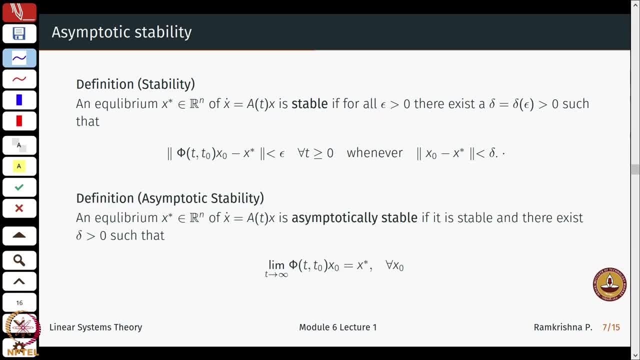 They would for. So the basic definition of stability should be satisfied. Now, additionally, on top of that, an equilibrium: x star is asymptotically stable. two conditions: One, if it is stable, and second, as t goes to infinity, x of t should tend to x star, which could be the equilibrium. 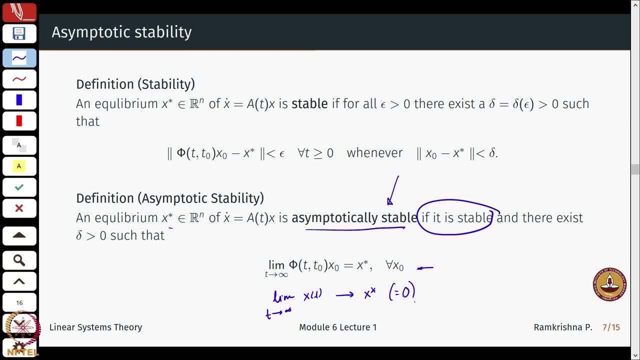 in this case for all initial conditions. So let us see what is new here. First is: so it means that, as t So suppose I am here, So this is my equilibrium. I say, well, I start from any point. I should actually eventually. 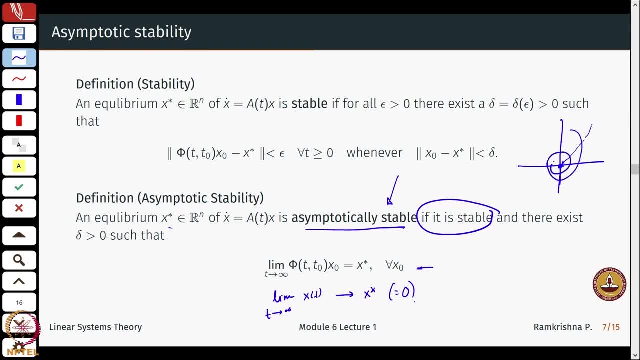 come back to this point. I can come back this way. I can come back this way, depending on the nature of the equilibrium point. ok, So this is what it means. Now, why do I superimpose A statement saying that stability is also a necessary condition? Why is it not always? 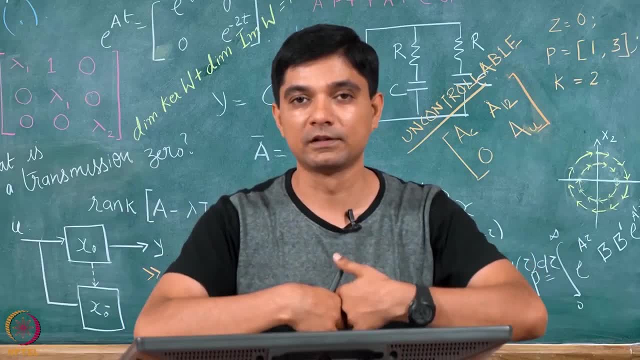 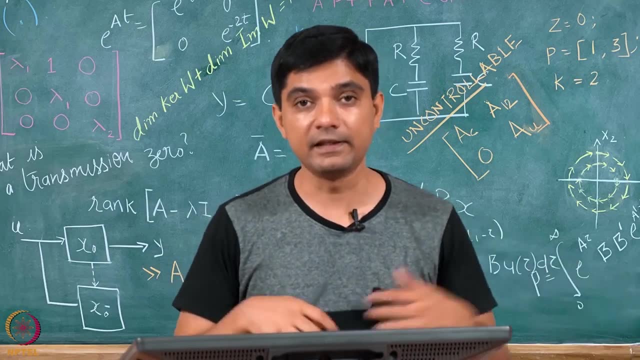 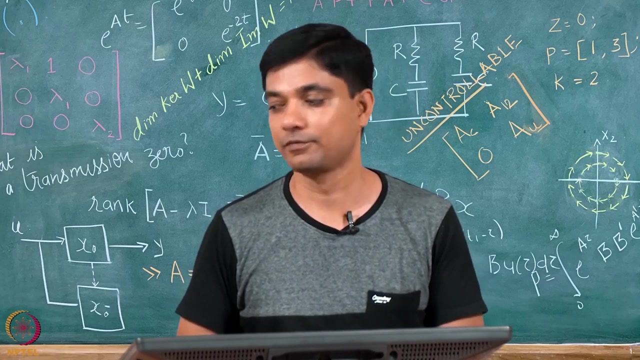 obvious that at t equal to infinity, I am going to the origin. So why should I additionally, on top of that, check for stability? ok, Let us do an example of that. In the linear case, it might like be obvious, but there might be some classes of systems which would behave. 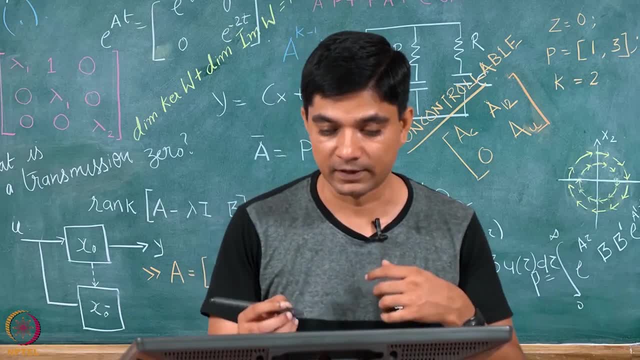 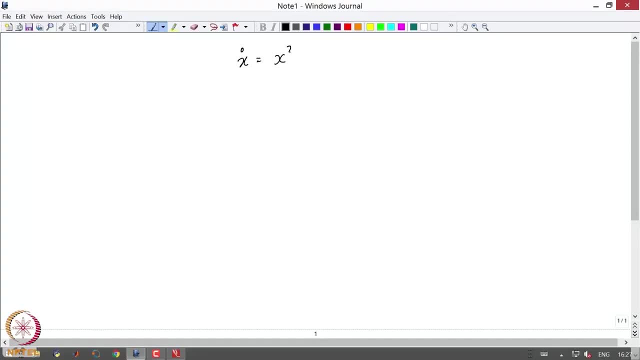 do an example of this. ok. So let us do an example of this. ok. So I have this system: x dot equal to x square, and let me say that x at 0 is 1. right Now, what is the solution? 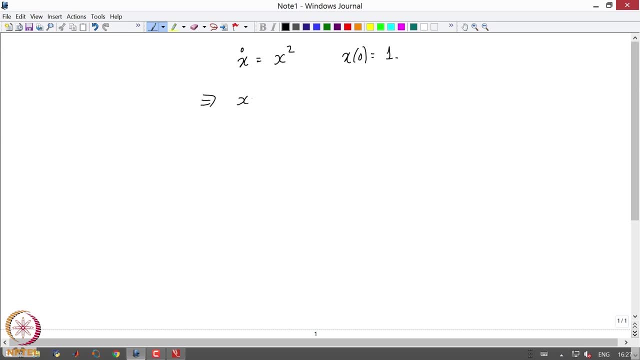 to this This: the solution turns out that x of t is 1 over 1 minus t. ok, So some strange thing will is likely to happen. 1, my system will say: start at say x 0 is 1, it will have. it will just blow up, right. So 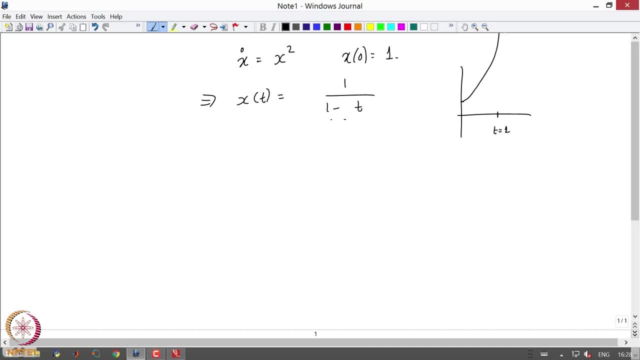 the value is not defined for t equal to 1 and you might think that well, it will actually come back after t equal to 1 plus and eventually, if I apply the limit rule, what happens? as t goes to infinity, this might actually come back to 0. I just draw it slightly better, right. 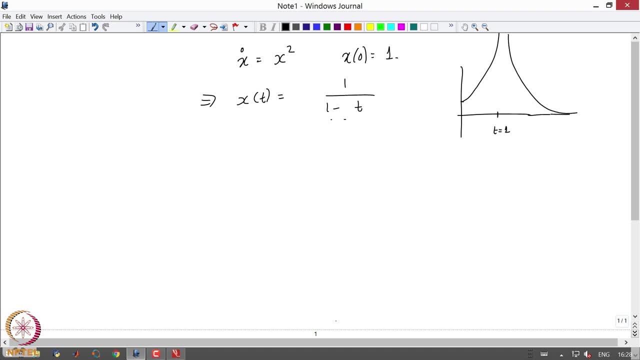 ok Now, is this a stable behavior? well, this is not right, because the solutions actually go unbounded. So what was the definition of stability? that, whatever the solutions do, they might just they should just be bounded by above from some, by some number? ok, This typically could happen in some non-linear systems and 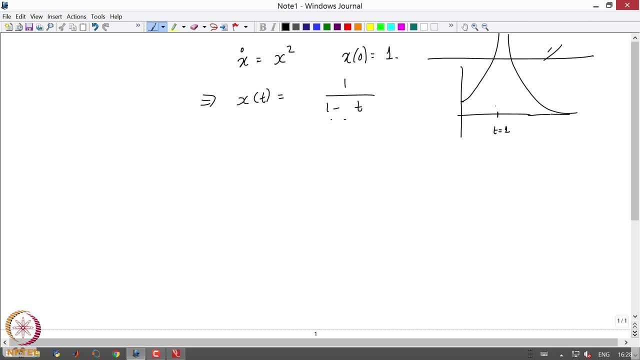 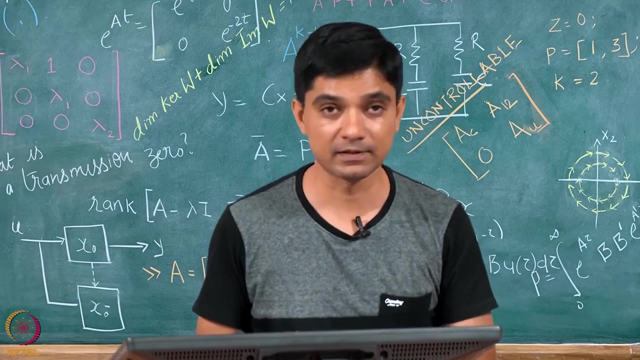 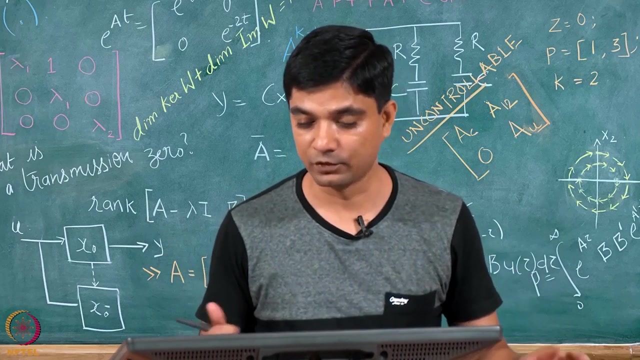 this phenomena, where at t equal to 1 the system blows up, is called the finite escape time. ok, Laurence K, Phenomena not usually, or almost never seen, or never seen in the case of linear systems, and therefore, to have a general notion of stability, we may have to impose this extra. 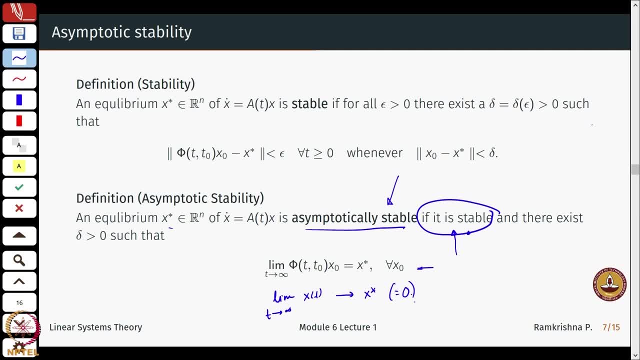 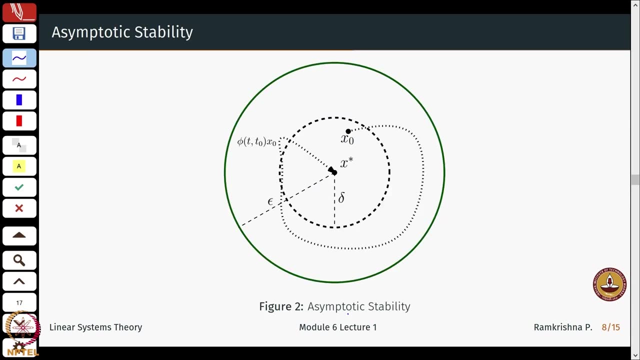 condition that first I need to check for stability and then I need to check what happens to the solutions as time progresses, what happens asymptotically to the system. ok, So I what does that mean that mean pictorially? I think they should now be like kind of kind of easy to visualize. 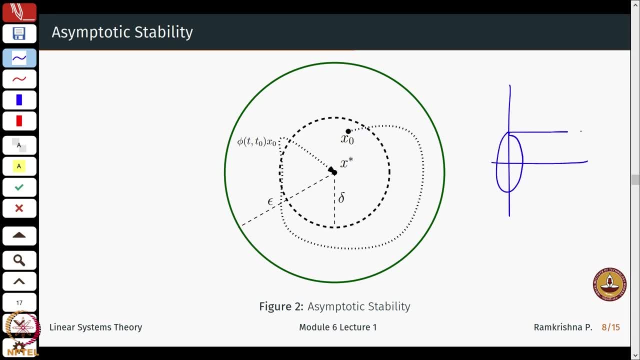 now right. So if I go back to drawing the cylinder diagram, start from any initial condition. I think that is nice way to look at it, is it just comes back to the equilibrium position. this is the equilibrium or x star. this is with time, ok. 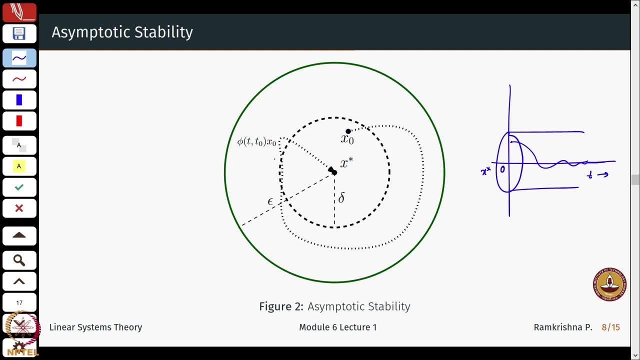 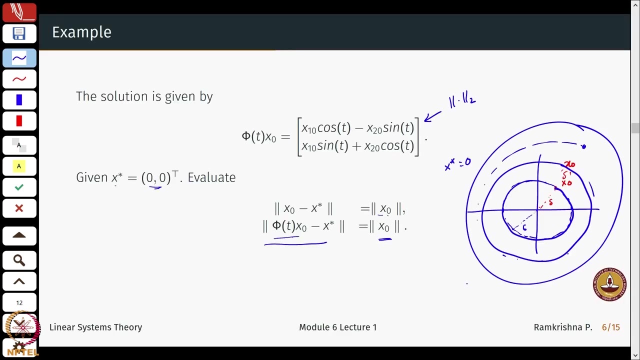 So, similarly here, I start with here, and somehow I just say at, so this is at, t equal to, as t goes to infinity. I come back to x star. ok, So that is, that is, this is stronger condition to check right. So, for example, is this system asymptotically stable? well, the answer is no. 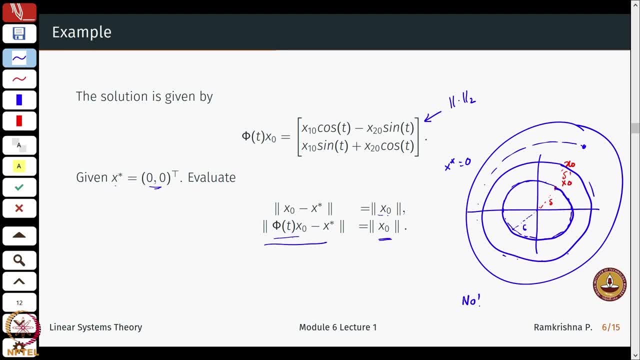 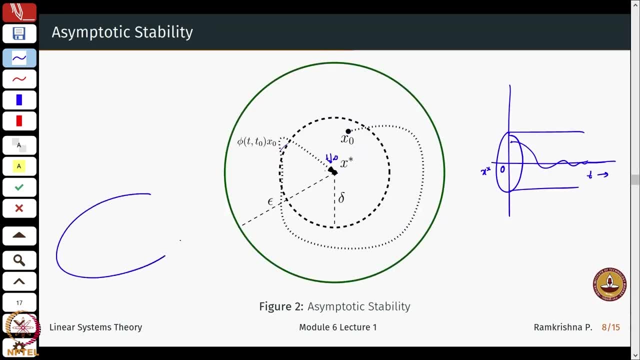 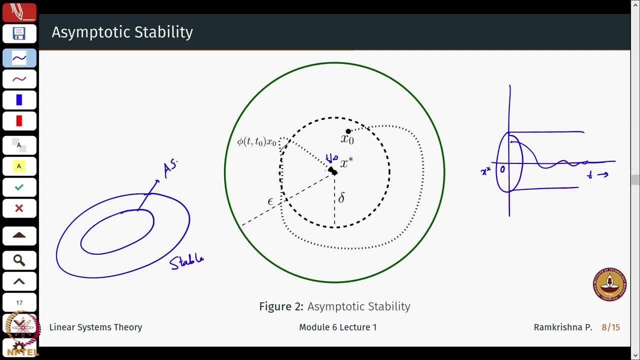 be asymptotically the set of asymptotically stable system. it is a stronger condition. So not all asymptotically stable systems are stable systems, but not all stable systems are asymptotically stable systems. So it is like if I were just to say asymptotically. 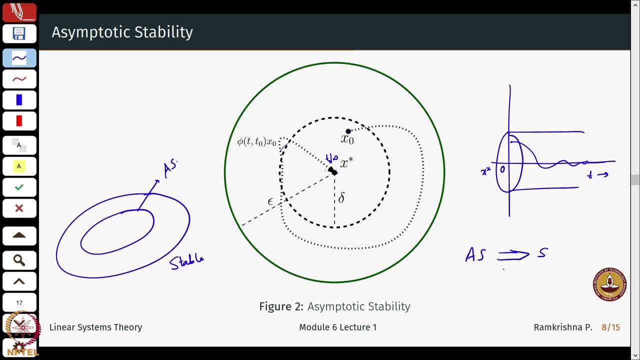 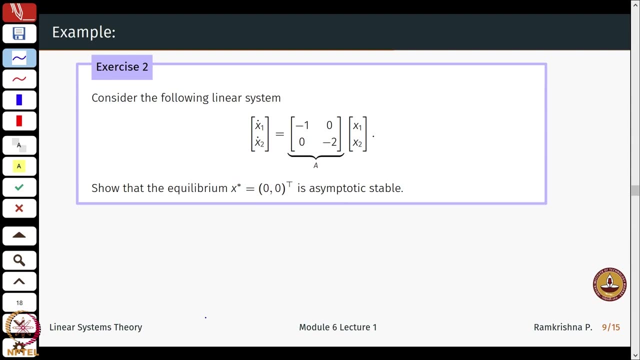 stable and stable. all asymptotically stable systems are stable, but all stable are not asymptotically stable systems. ok, Just a little little counter example to that. is this what we saw just now? ok, So let us do again. seemingly simple looking example. if I just were to ask you to compute the state transition matrix solution, it will. 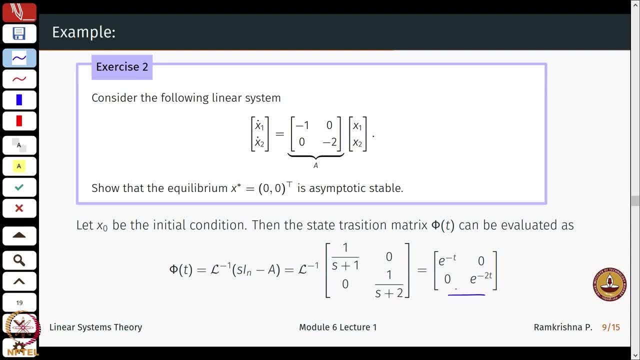 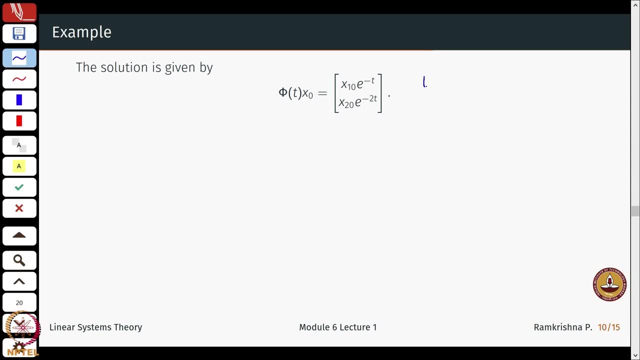 be like by heart right, because it is in the diagonal form. and then the e power, a, t, is easy to compute. Let us say I start with certain initial condition: x 1 naught. x 2 naught. again for simplicity, I assume t naught is 0.. First can I check for stability. that will be easy. 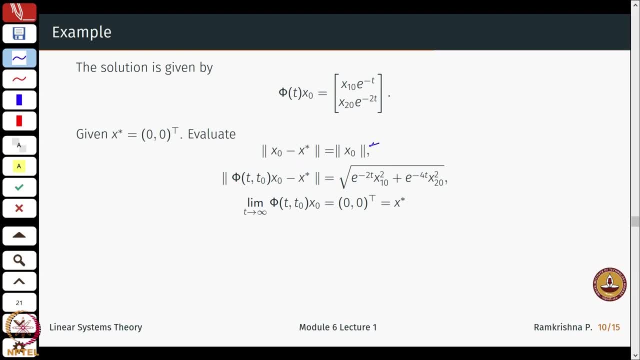 to check right. So this is my, the delta ball. this will be how the epsilon ball would look like. So the first two conditions will tell me that the system is easy to compute. So it is stable. ok, Now how do the? so I can actually find the upper limit of this right. 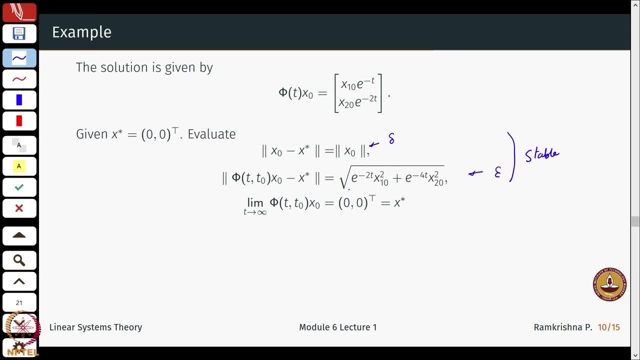 So I will just leave that as an exercise. but what? look at this expression here. what happens? it has two times, two terms which are, you know, exponentially decaying, right, and therefore, if I put the limit as t goes to infinity, I will just end up here, right? So 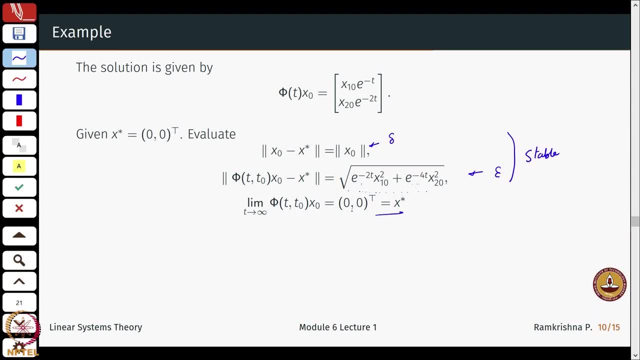 limit. t tends to infinity. phi t, t naught x naught is 0.. is the origin, which is the equilibrium of interest. Again, simple example, but good enough to verify what is happening here. ok, Is that? are we happy when we say this? this is just. 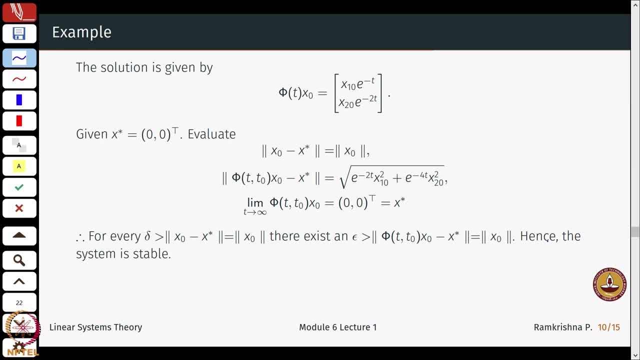 a statement which concludes that the system is the first that this system is stable and second, that this system is also asymptotically stable. right? So just repeating that and writing down that formally. ok, So are we happy with this? Well, one may ask. 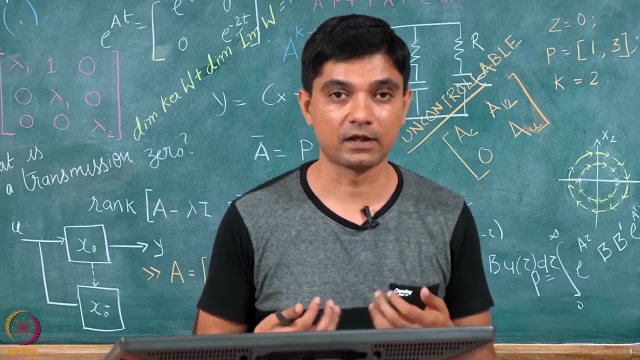 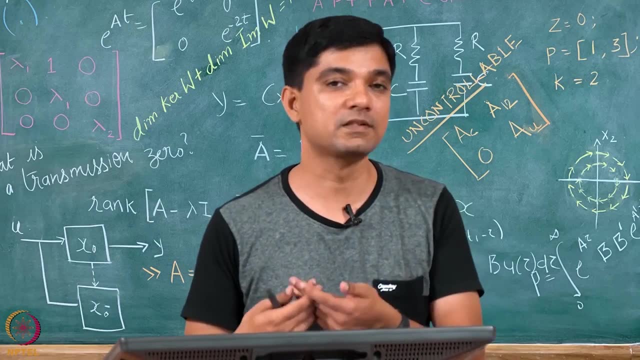 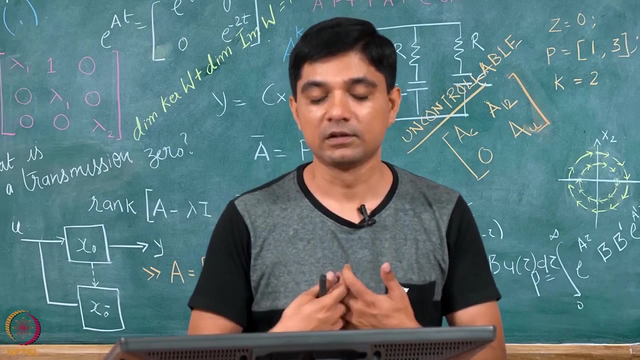 how fast are we coming to the origin or how fast are we converging to the equilibrium point? So whenever I say origin, it is also means it also means the equilibrium point. So these things will be used in the equilibrium Interchangeably: origin, the equilibrium, and so on. So I would also want my system say: 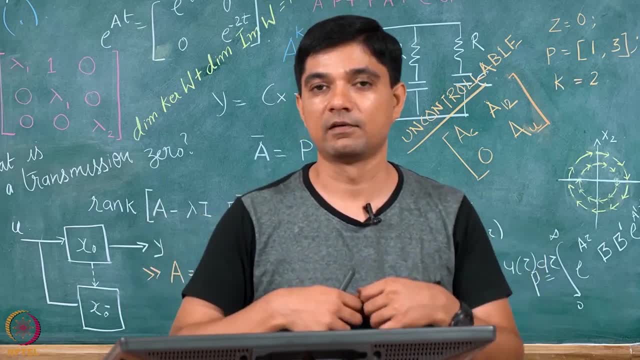 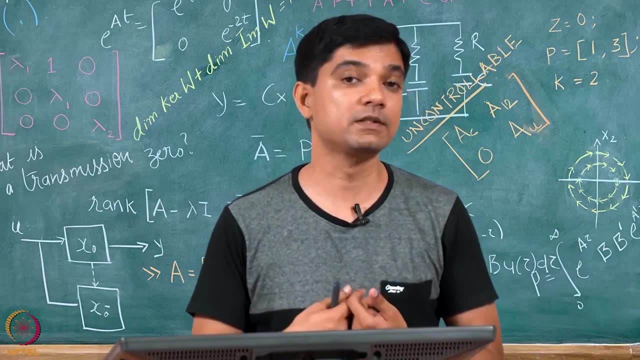 for example, it takes forever right If it is a, if it is a very heavily damped system, maybe the response is very slow And therefore I would also like to see what is the rate of convergence to the equilibrium point, And therefore I need to define further a stronger 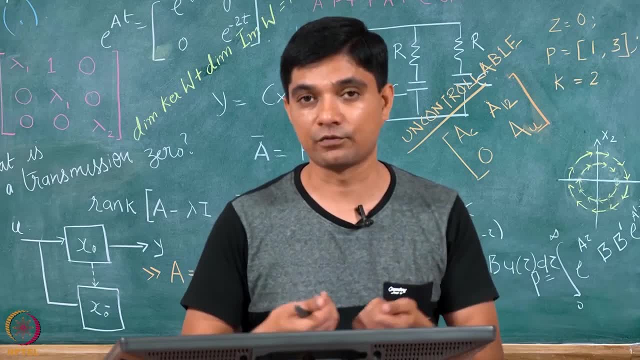 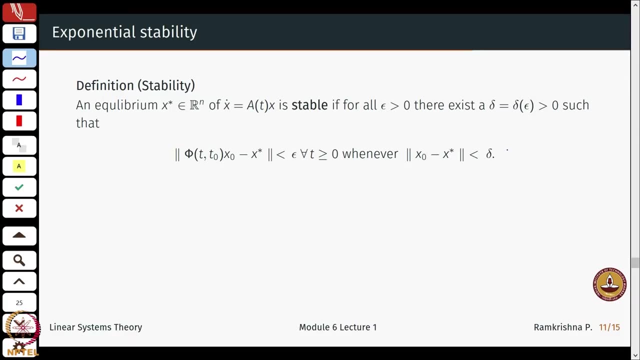 notion or do I, can I quantify the rate of convergence? and that is where convergence comes in. the notion of exponential stability: ok, What does it mean? Again, the basic thing is to look at the definition of stability. ok, When is the system additionally exponentially stable? Of course, first I should check if 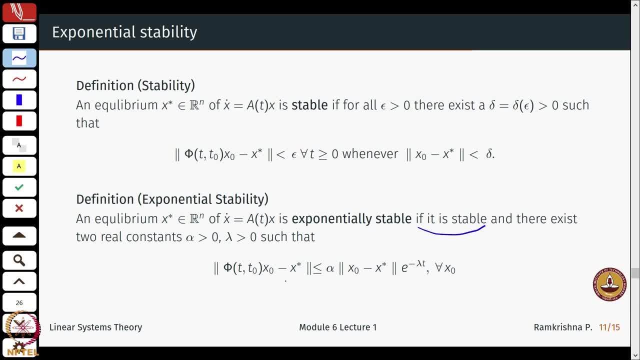 it is stable or not, and then there exist two constants, alpha and lambda, such that something like this holds: ok, What does this mean? Say suppose I have a solution which starts from initial condition, it goes whatever, like this, like this, and maybe eventually goes to the origin, Now exponential. 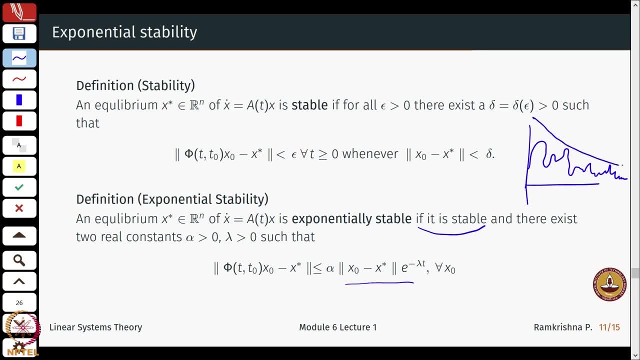 stability would mean. can I actually bound this from above by an exponentially decaying curve? right? So this is exponential decay, right? So if my solutions are always under an exponential curve, is called an exponentially stable system? Mathematically well, this is an exponents. my 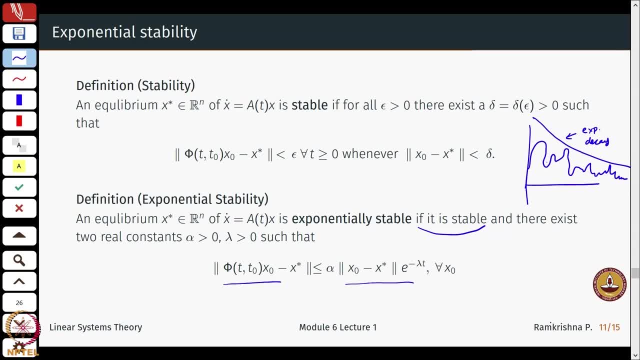 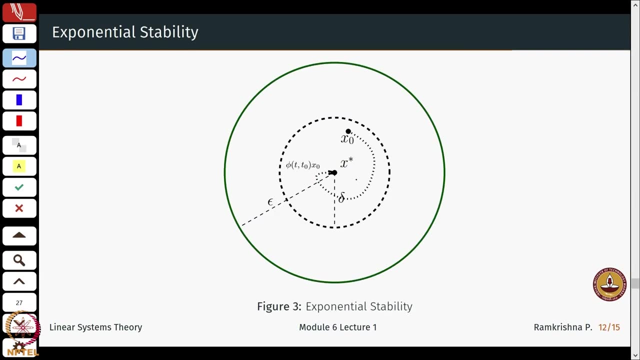 solutions. So this is my solution- is bounded by an exponential function, and this is exactly what is written here, right? So this is this will be called the decay rate, and so on, right, ok, So I can just write down a picture which looks like this, but I think it is easier. 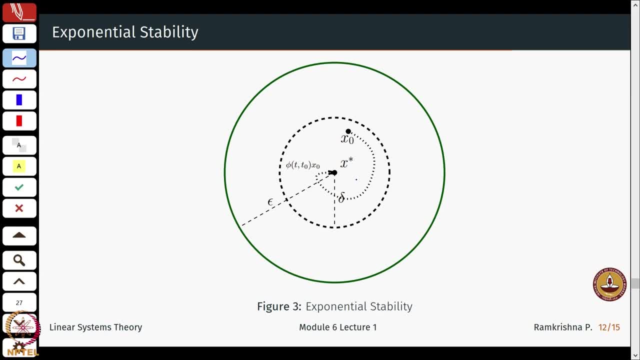 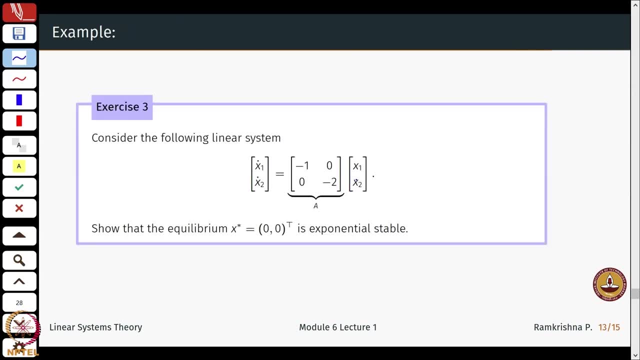 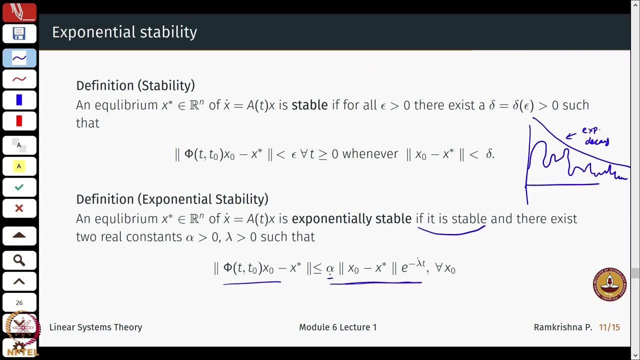 starting from what we know earlier, it is now easy to interpret this picture. ok, Again, I come back to this system Now. I want to verify if this is exponentially stable and then, if it is exponentially stable, what could be the values of this alpha and lambda? ok, I will. 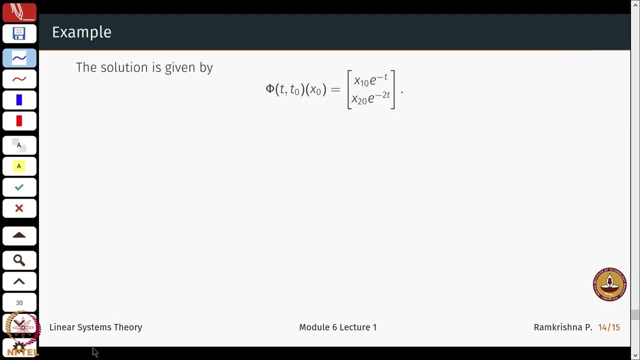 again. skip the initial condition, skip the little computations again. t naught could just be the t naught equal to 0, ok, So again, this is. this is from previous. So what is the solution? satisfy phi, t, x naught minus x star is just bounded by e power minus t, So it decays. 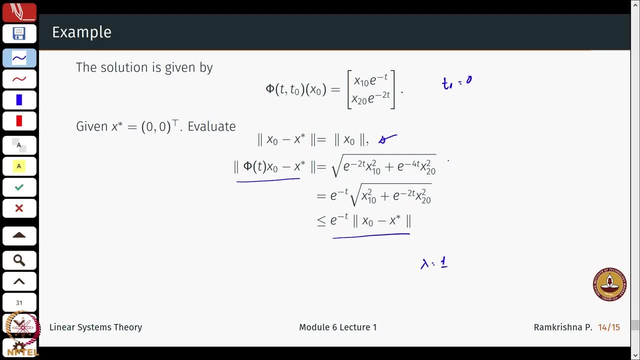 at a rate of lambda equal to 1. ok, So this three steps can be can be easily verified. I am just computing the two norms here, So that should be easy. Now. so far, well, we know that this is stable. Something inside could be asymptotically stable. it's a smaller subset. 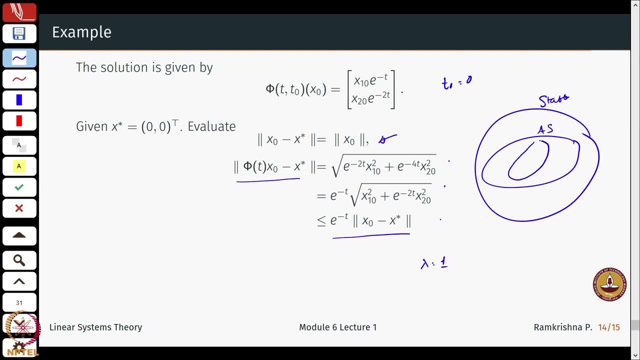 and exponential stable is even a harder condition to check, right? So therefore this is, the strongest condition to check would be that of exponential stability. So stable is just is a bigger set. asymptotically stable systems are stable. exponentially stable systems are. 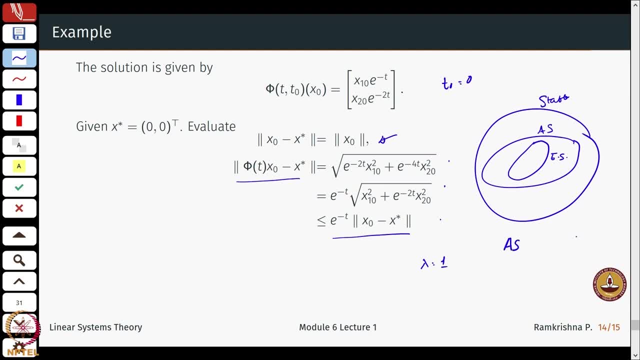 asymptotically stable. So now relation between asymptotically stable and exponentially stable. All exponential stable systems are asymptotically stable, but are all asymptotically system, asymptotically stable systems exponentially stable? Well, it turns out in the LTI case, which means the 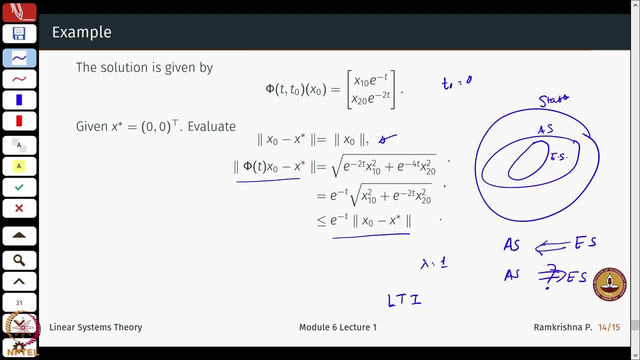 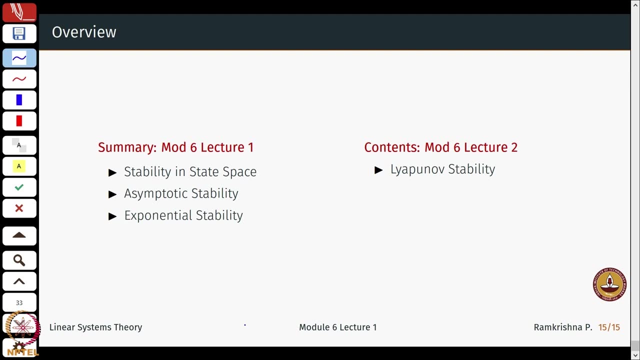 linear time, invariant case. exponential stability and asymptotic stability would actually like coincide right, and we will do proofs of this. So I just conclude today by just introducing to you the three notions of stability: The basic definition of stability, asymptotic stability, which is a stronger version, and something which also tells us the rate of. 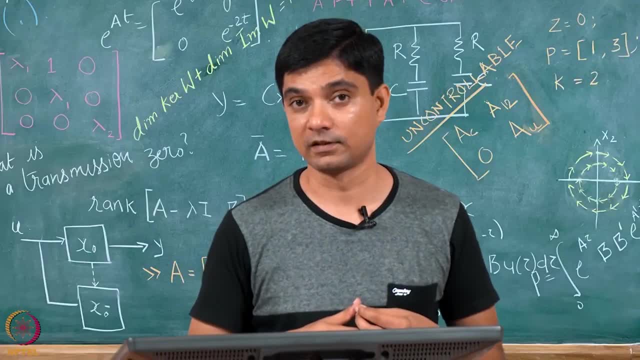 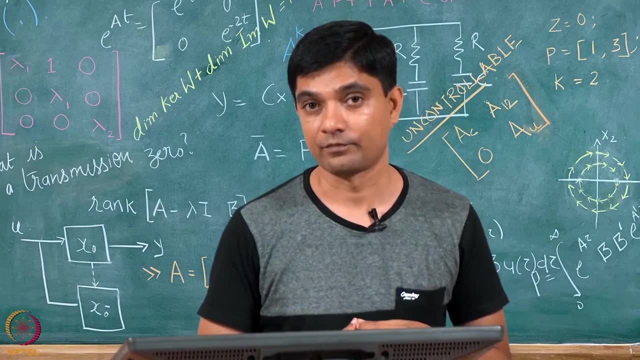 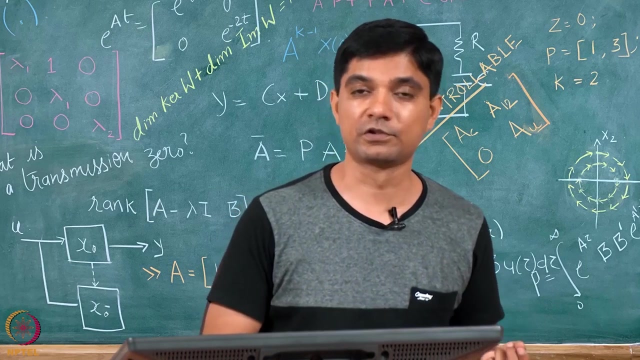 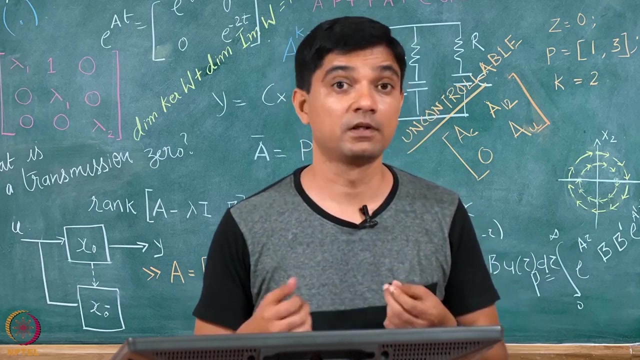 convergence is the. is exponential stability Now, given a system? now how would I verify stability? Say, I am given system in R 4. Now can I all the time compute the solutions, compute this constants, alpha lambda and so on, or compute various norms that may not always? 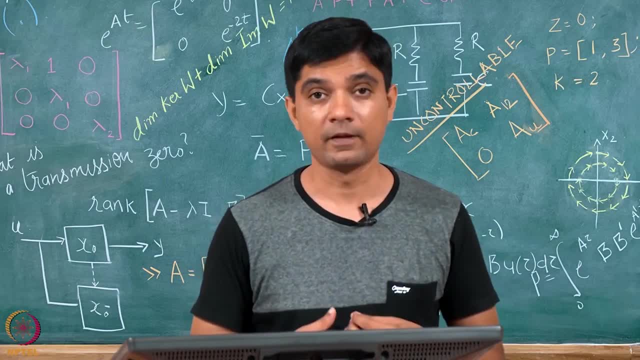 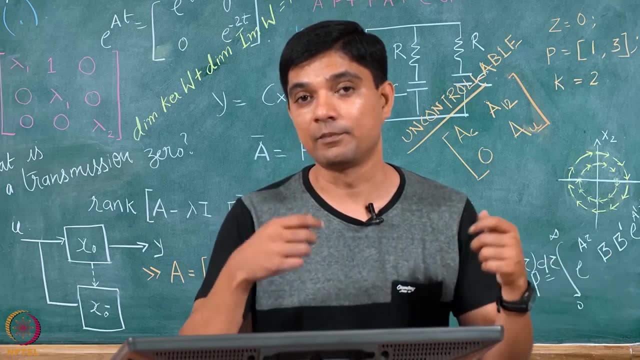 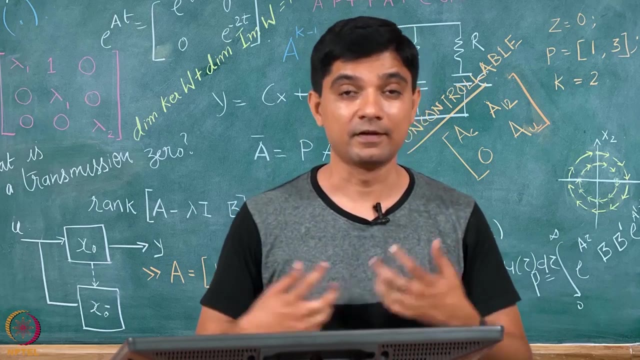 be easy Now. are there effective computational tools which will help us verify stability of systems? Similarly, in the transfer function case, we do not really compute the check if the Impulse response is absolutely integrable or not. right, We just translate that to an. 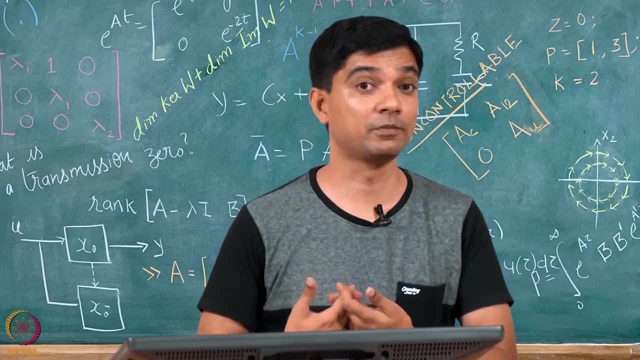 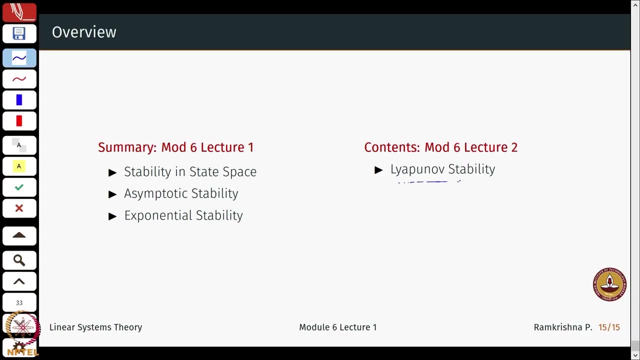 easier way of verifying, which is with respect to the poles. Similarly, in the state space methods, we will next look at the notion of Lyapunov stability and identify tools which will help us verify stability certificates for LTI systems. Again, much of the tools that